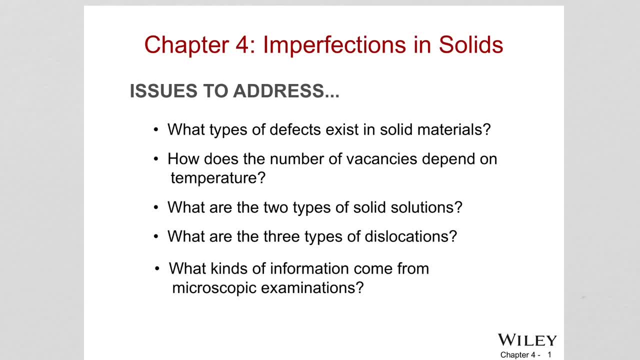 And we're gonna see what is a solid solution and what are the types, What are three types of dislocation. So we're gonna towards the actual solid solutions. So we're gonna talk about what are different types of list to be in them. So we're going to. 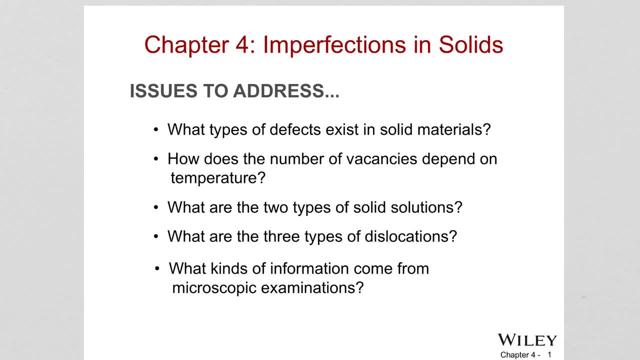 see, dislocations are line defects, linear defects and it's a very important defect in the structure and we're going to see what three types of dislocations are and you guys need to do some visualization to understand that and we're going to take a look at what type of microscopes are there and what type of information. 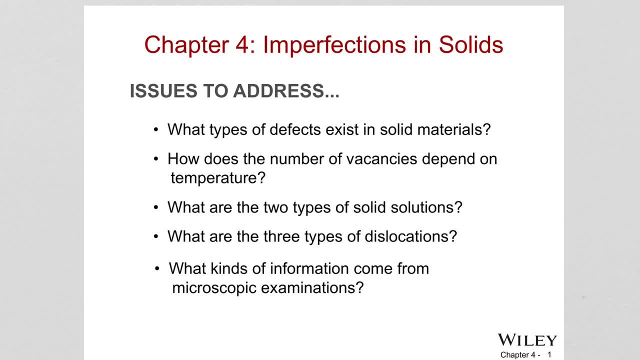 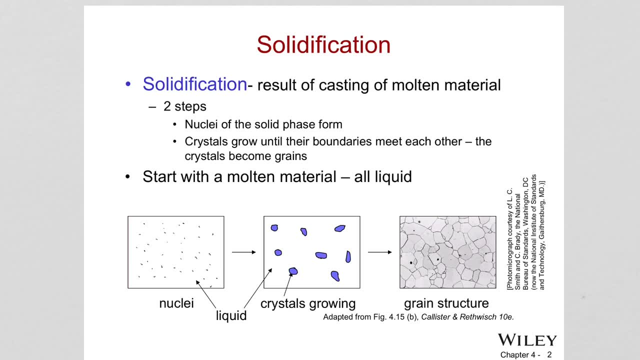 we get from microscopes. so always when we are processing a material, we start with solidification. right, we have a molten metal and we need to shape it. therefore we do casting and the material needs to solidify. so during this solidification, several things takes place. first, from the liquid, 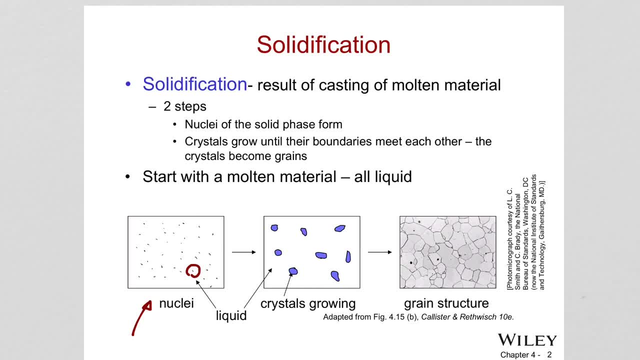 nucleoids gonna form tiny solid particles, atomic size, nano sizes, right, and gross micro size. and what happens here is, as the solidification continues, as we decrease the temperature from the molten state to a solid state, solid state starts to form from the liquid and we can see that from the nuclei. then 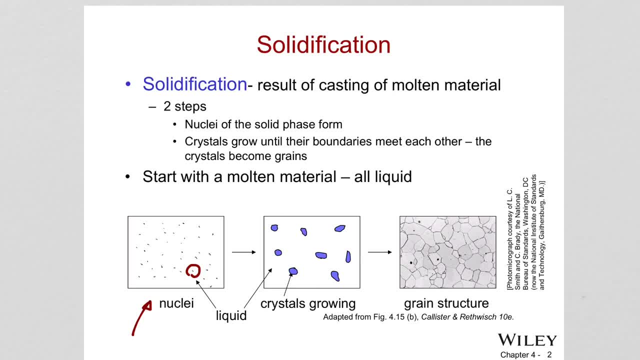 more atoms come together, forming the crystals. as you see, the crystals are growing and then at the end we have a grain structure like this. so all these lines are the grain boundaries we are seeing, where atoms within those regions are ordered in a certain directions. so those grains 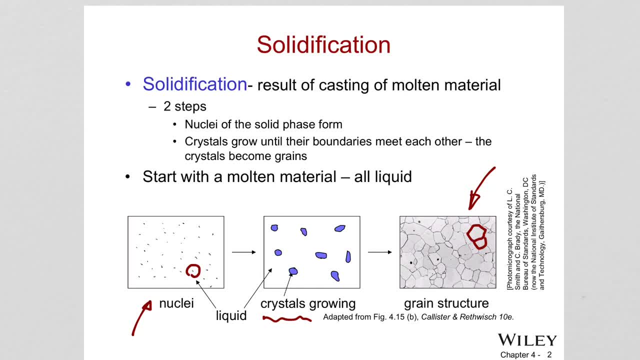 actually we're going to see. the grain boundaries are two-dimensional defects inside the structure. so when we say defects, there is something like uh, understood, like this is something negative. defects can be negative, but also positive. they can be intentionally introduced into the structure like semiconductors, where we intentionally introduced 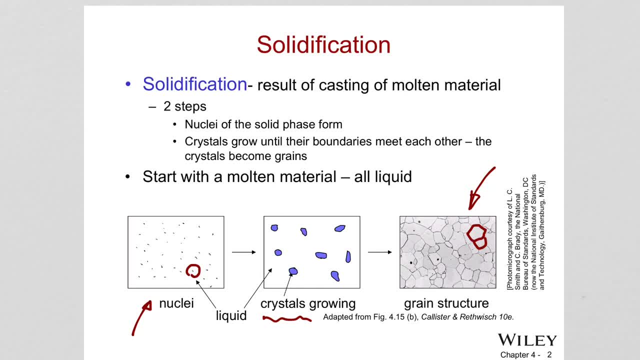 certain elements to manipulate the conductivity of the silicon, manipulate the conductivity of material. you can do that intentionally or, for example, in this case, grain boundary control is important because it is a way to strengthen the materials. we're going to learn later. okay, so not uh. when we say defects, don't think about it as something negative and understanding how. 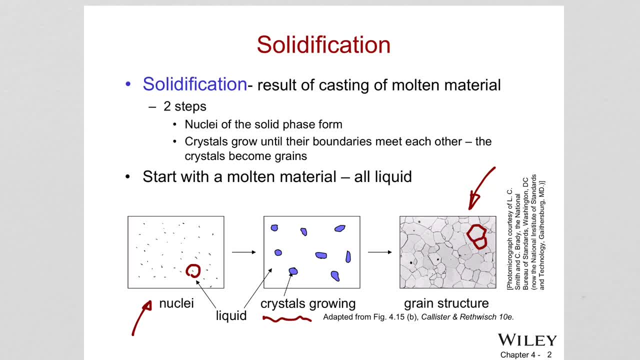 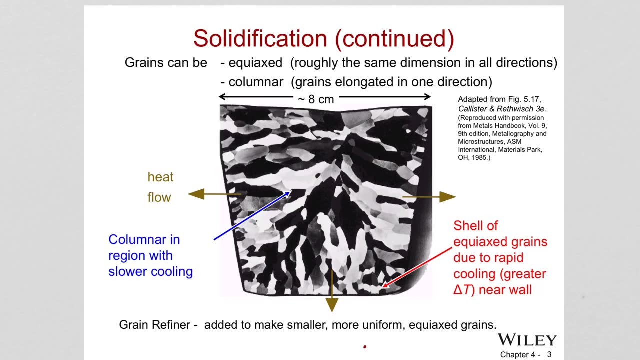 defects affect the properties and how we can control them, shape them, will help us to manipulate the properties of the materials. so, during solidification, for example, all the factors will affect the grain shape, for example. of course the is. so if this is our mold, we are doing casting right. and when we dump the liquid, 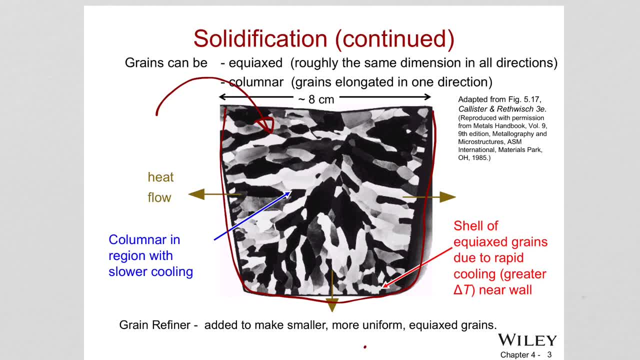 uh, molten metal. it is now solidifying and during that grains will form. but grains will be affected with the direction of heat flow because the material is going to lose heat to the environment in that direction. as you can see, the grains are forming this aligned shape along the heat flow. 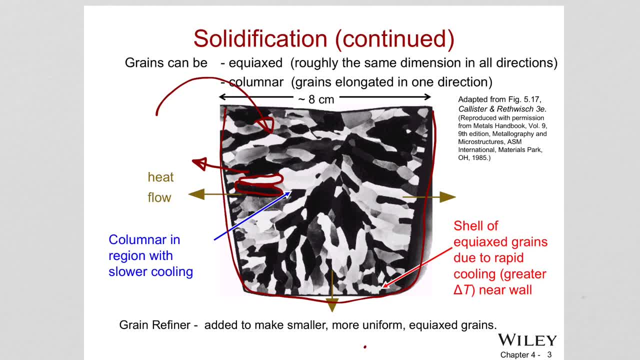 direction. okay, so we call these columnar grains. so this is just to give you an example of how defects are important. okay, the grain boundaries are defects, so grain size, grain shape is changing, so these are columnar grains, but within very close to the, actually the mold itself. okay, here, because they are in direct contact with the. 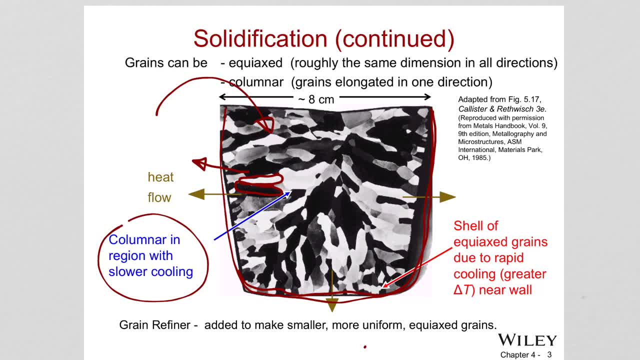 material, they will cool very quickly. okay, so this place, this region very close to the mall, it will create a quick shaped grains due to rapid calling, which is near the wall. so, as you can see, it is not easy as we imagined and things depend on many other factors in this. 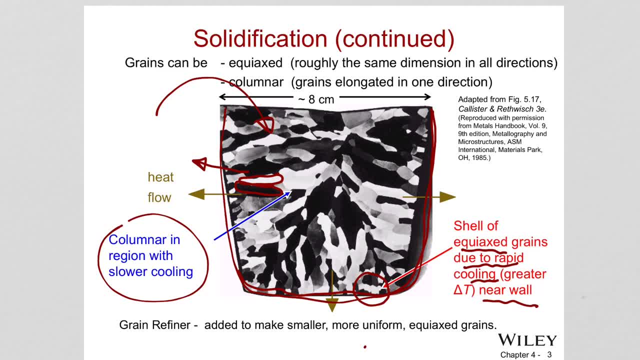 case how the heat flows, how the material cools down and you can even see some shrinkage here. you can see right, because when we are soool the heat falling 2021 width line, we are waiting. we going to begin to shrink down the Gleich кровly~~. 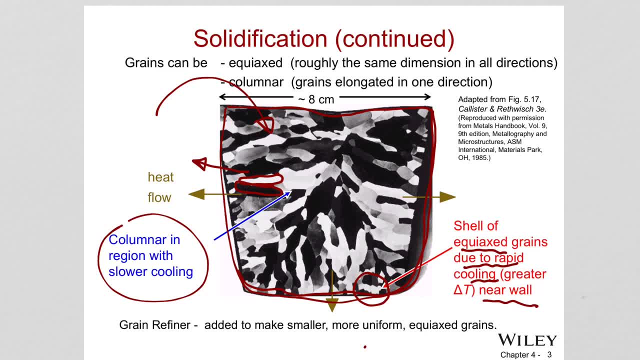 solidifying material also shrinks. so people wants to obtain small grains, equix grains and uniform grains, and this is done because a materials have showing more strong properties. they are acting more strongly when we have equix and small sized grains and we're going to understand. 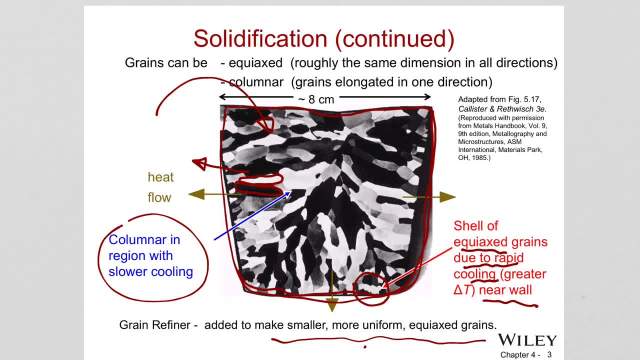 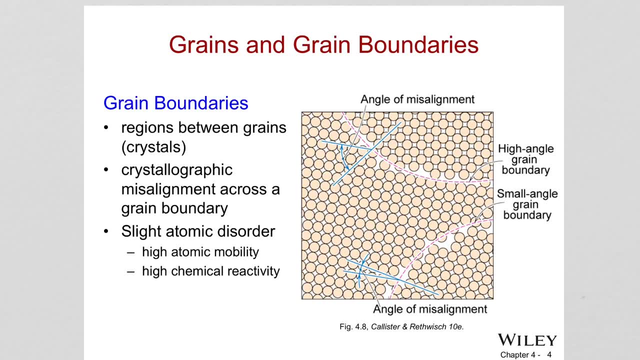 what are the reasons behind that? okay so why grain and grain boundaries there's are defects? basically because there is, when you look at each grain and when the where they're actually getting together, there is a misorientation, misalignment. okay so, so we have seen. for example, I told you guys, grains are different regions where atoms are arranged in different. 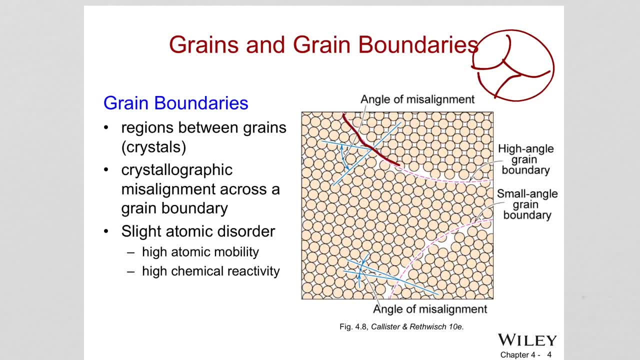 orders. you see that here in one grain- this is the grain boundary, boundary in between the grains- the atoms are aligned in this direction right, and if you take a look at another grain, it's like that in reality. of course, when this direction changes, there is not like a visual. 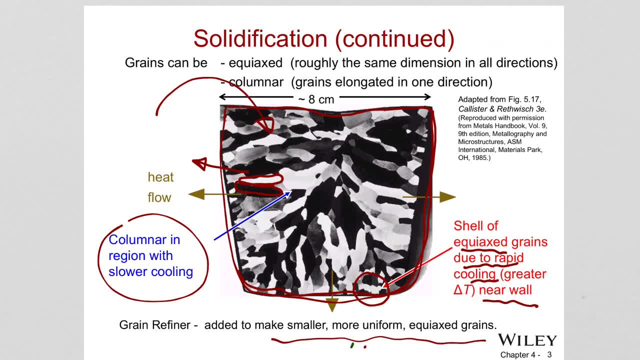 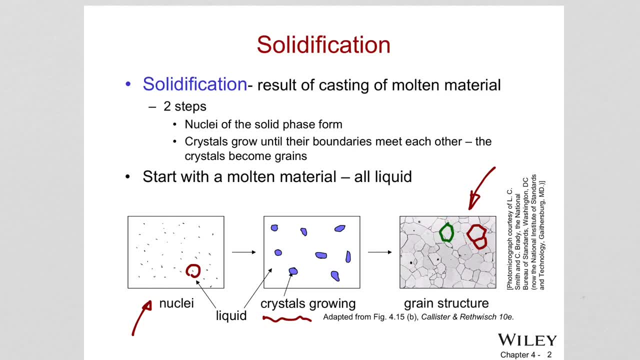 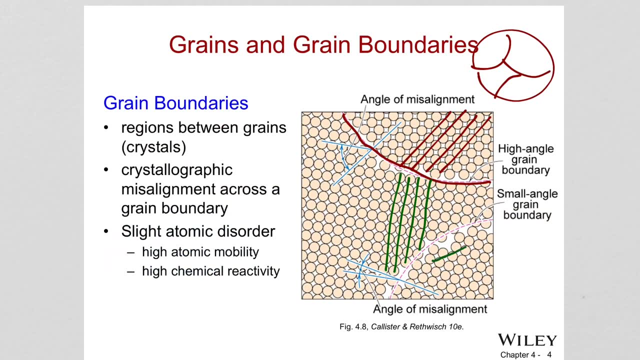 grain boundary. Yes, we are seeing in the microscope like this visually. the reason is because these materials are etched with acids. since there is misorient, there is a randomness, more random arrangement, as you see along the grain boundaries. there is a randomness if they are not arranged in. 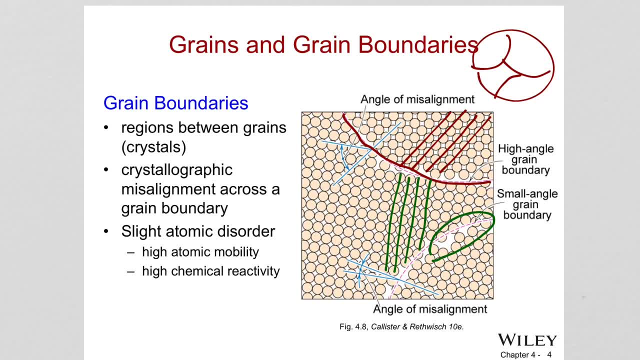 a perfect order. that's why this is defect. grain boundaries are defects. Yes, because they are not arranged in a perfect order along the grains, and that's why they are more reactive, because they are not stable like this Adam. right, this Adam is connected from every direction and it is very stable, but this Adam is more free. 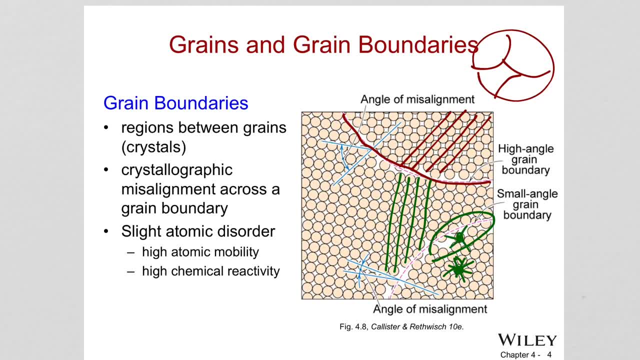 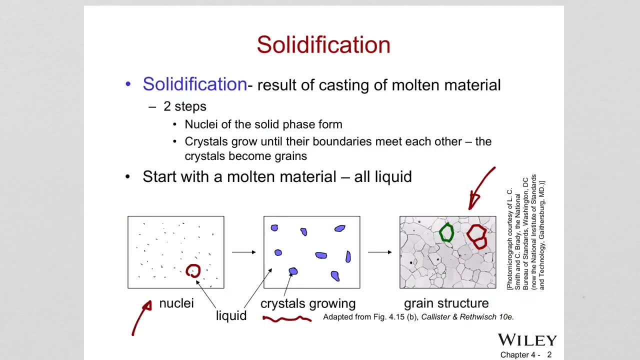 So it wants to like everything in the nature. it wants to be more stable. therefore, the grain boundaries, atoms, near the grain boundaries they are more reactive. that's why when they with acids they react and that's why optical properties along those grains changing, they scatter the light differently. that's why we are seeing actually solid lines in them under the 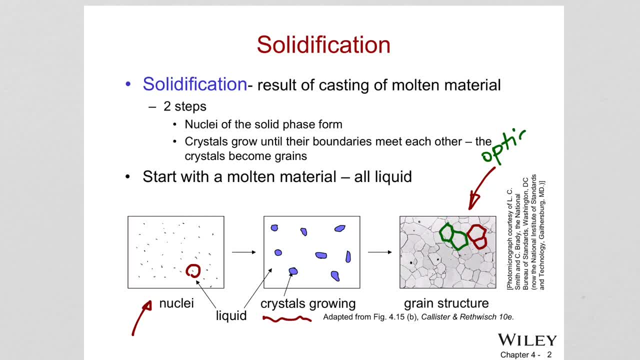 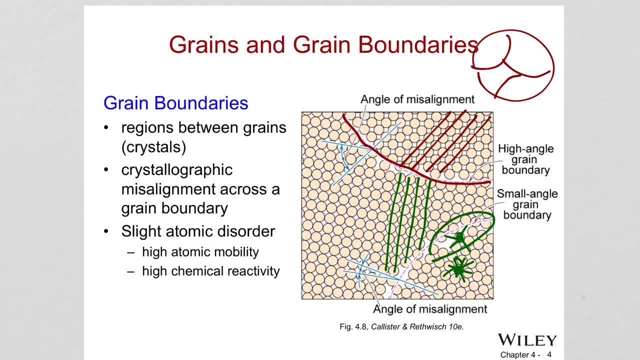 microscope. so this is an optical microscope image. okay, so in reality, of course you are not seeing line. there are no lines like this. of course we are imagining there are lines and there is just a change in the direction of atomic alignment. okay, so these are aligned, for example, in this: 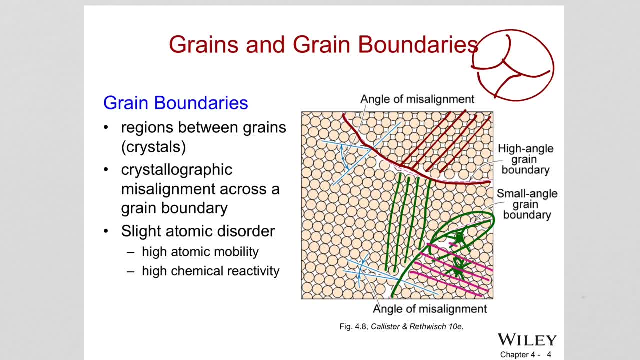 direction. all of them different. okay, so crystallographic misalignment across a grain boundary. that's why we call them defects, because the atomic arrangement is random and grain boundaries are the regions between grains, as we talked about them. there is atomic disorder when we are crossing the boundary. okay, this, of course, creates atomic mobility, if they 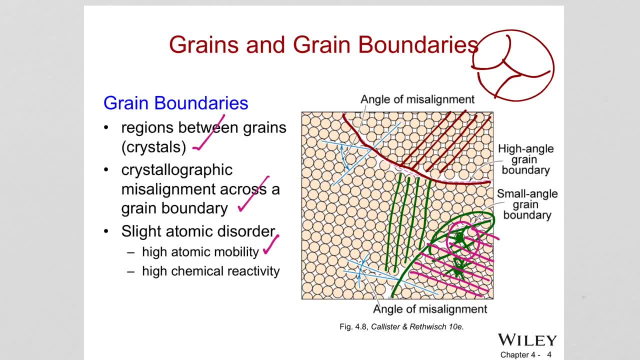 are more free. as I said, they are not bounded in all directions. they are more free and they are more reactive because they want to react with something and become stable. so they etch them with acids well before putting under the microscope so we can see the actual grain boundaries and, of course, depending on how, what, to what degree this. 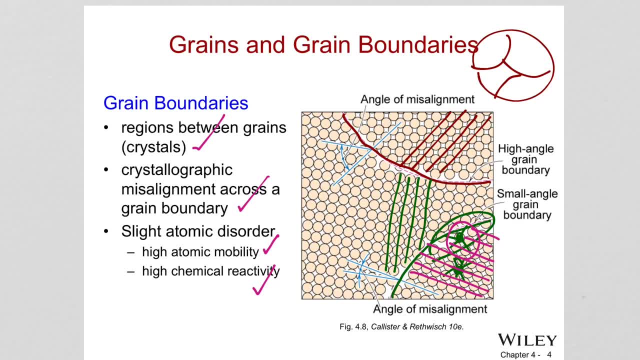 alignment changes. you can call them high angle grain boundary or small angle grain boundary. as you see from here we are like this and this is the continuation, but alignment here of the atoms is like that or another direction, it doesn't matter. so there is a change in this, this much. 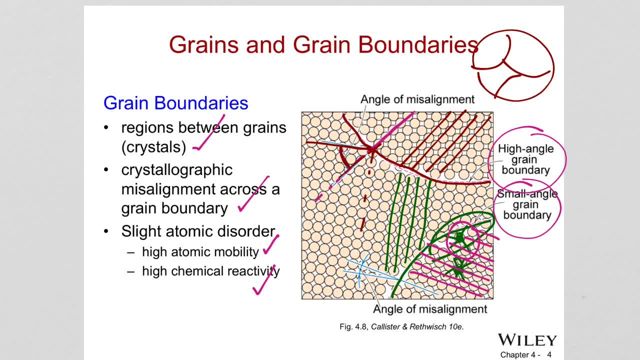 angle. there's a change in this much angle. there is a change in this much angle, there is a change okay. or like this: so there is an angle, and if it's big, this we call it high angle grain boundary- okay. and if just a small change in the alignment, like this, this is small angle grain boundary- okay. 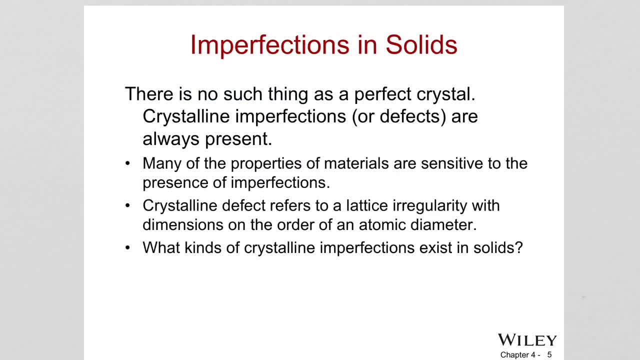 that's it. so this was an example, and now let's look at what type of imperfections are there in solids, in, if you want to categorize them, and we said, there is no perfect crystal and defects are always present in the structures and many properties can be changed with the 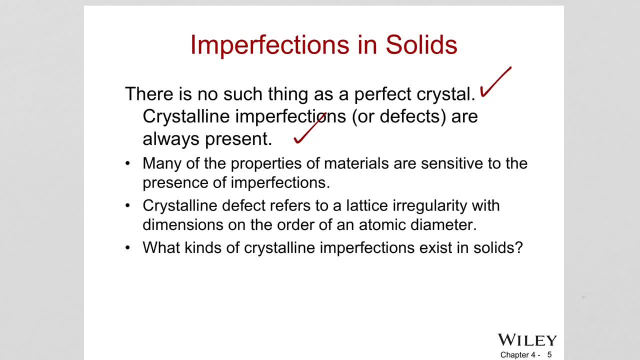 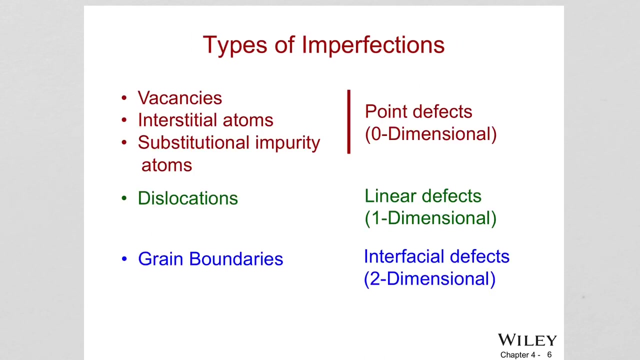 addition of or removal of the imperfections. the properties are very, very sensitive to the presence of imperfections or defects and we also said these are lattice irregularities on the order of atomic diameter, so very small. okay. and let's see what kind of imperfections or defects exists in solids. so types of 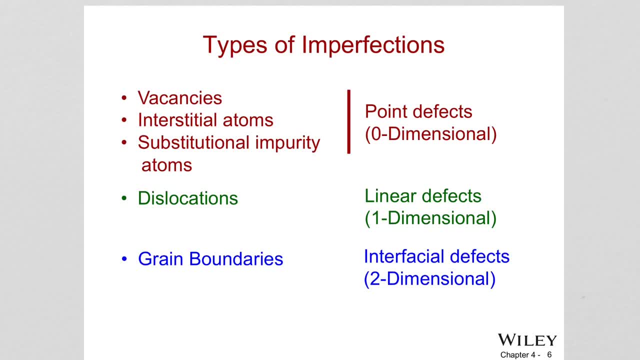 imperfections, we categorize them based on their dimensions. so zero dimensional defects are called point defects. so egg no, XYZ right. so linear defects: they are one-dimensional, they are linear, and there are grain boundaries. grain boundaries are two-dimensional. okay, so think about each grain boundary. of course we are. 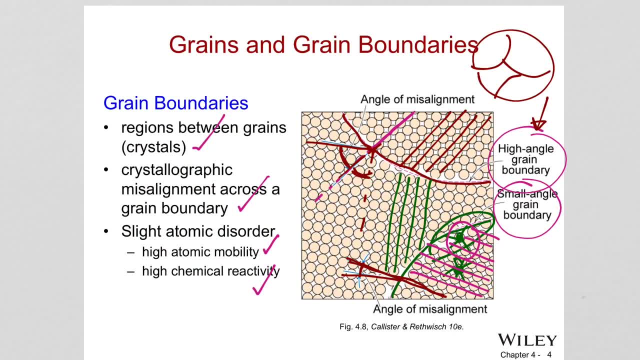 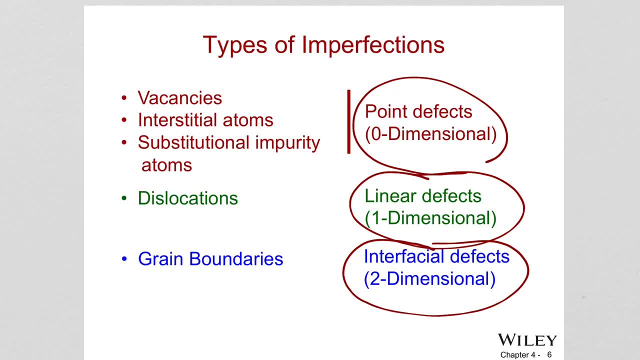 seeing here. think about this is happening in 3d space, right? so there are two-dimensional defects, the surfaces in between two spheres. think about it that that the campuses in between the spheres are place these two spheres right here and the two spheres are at the same place. 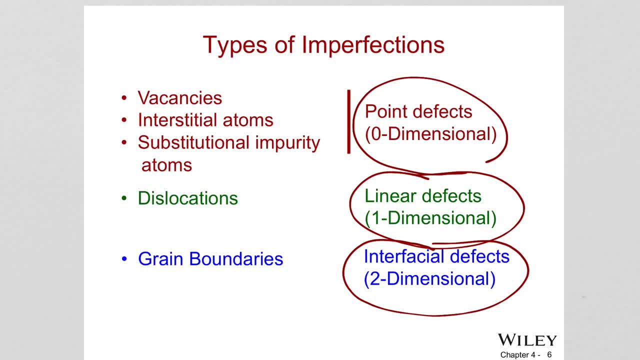 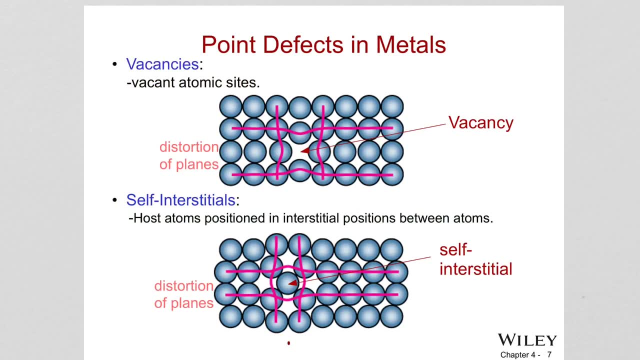 so let's see, the simplest form of point defect is a vacancy. it is basically, as we can see, it is basically a vacant lattice side. okay, so we see that their atoms are packed in a certain arrangement, but then the atoms are packed in a certain arrangement, but then the atoms are packed in a certain arrangement, but then we have a them in any way to make the potential verb to be categorized. primero la libertad. 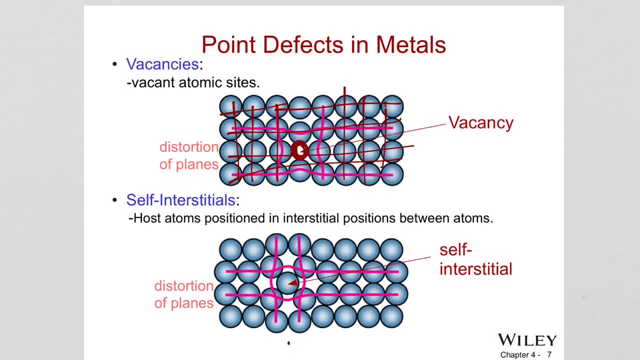 One atom is missing from here. It's gone And it creates, of course, the whole lattice. It creates distortion along the whole lattice, Whole crystal structure, because I mean the nearby structure, of course, nearby. If you move far away from this vacancy, there is going to be perfect order again. But close by nearby of this vacancy site, there will be distortion of the atomic structure, atomic planes And basically vacancy is just a vacant atomic site. One atom is missing. It's supposed to be there but it is missing In a perfect order. It has supposed to be there but it's missing. 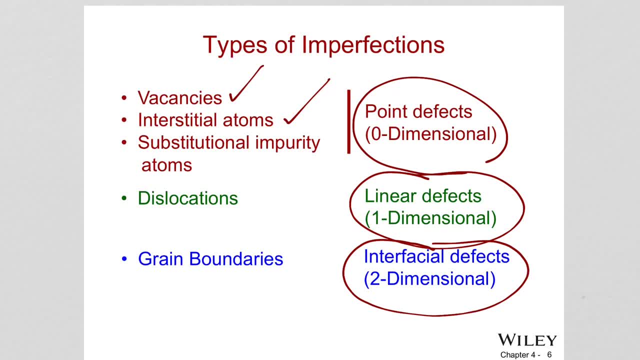 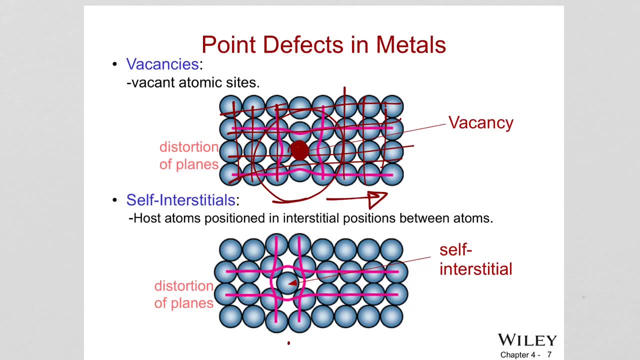 And there are interstitial atoms. Let's see Interstitial atoms. they can be self-interstitial, as we are seeing here. So when we say interstitial, when atoms pack, they have empty regions in between them. We call them interstitial sites. So atoms pack. 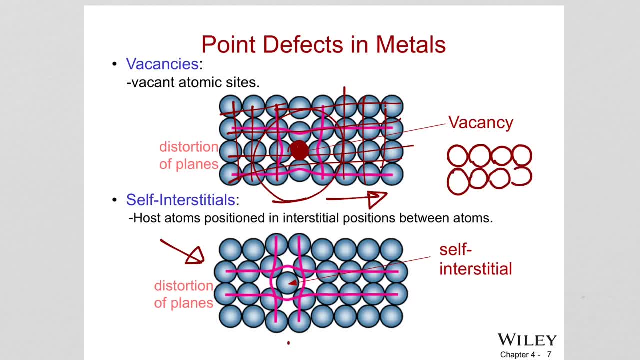 So atoms pack like this, Right In a perfect arrangement, In a very high packing arrangement, But you see, even if we want to pack them very well, So this is not the perfect packing. actually, Perfect packing is FCC, Right, It was like this: 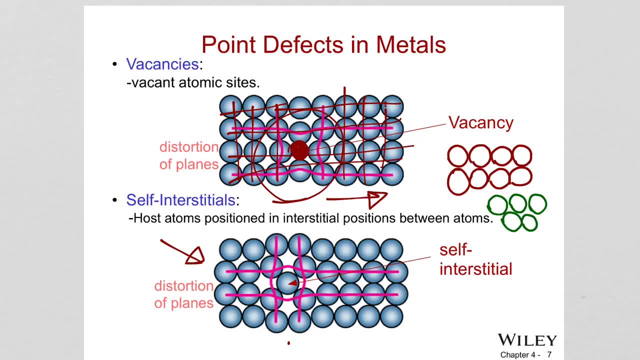 Even with that, there is going to be empty regions in between the atoms, And we call this. they cannot have no empty space. So these are, These are called interstitial sites. So what could happen? Adam itself can go into this interstitial site and we call it self-interstitials. 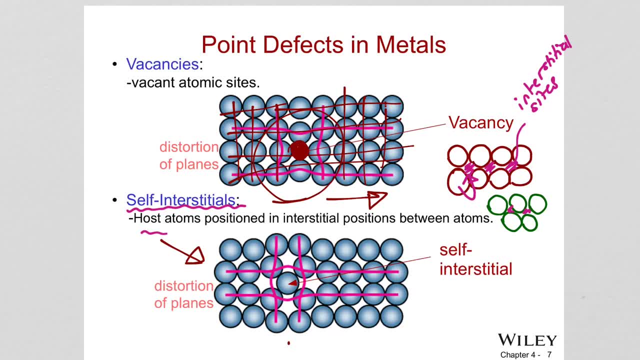 So if you look at this figure here, it says host atoms positioned in interstitial positions between atoms. right, so blue, each blue, is the atom, but an extra atom which is getting into the interstitial position here and of course that create a lot of stress around it because it is pressing on the surrounding atoms. it is not. 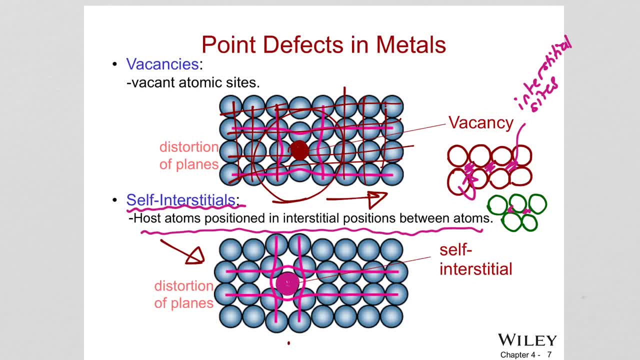 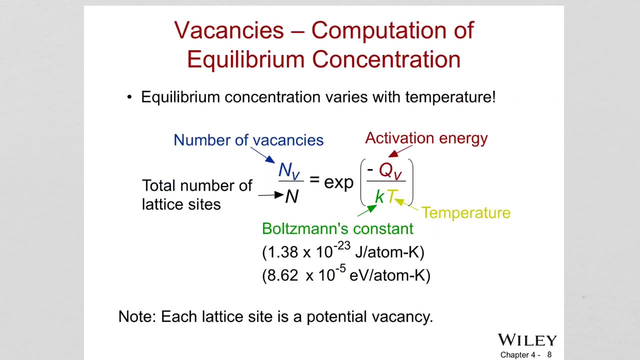 its correct plates. it's too big for that interstitial side and very close by around it it is causing stress and distortion in the lattice. okay, then we call this self-interstitial. so thermodynamically all materials has to have vacancies. but because it is shown that 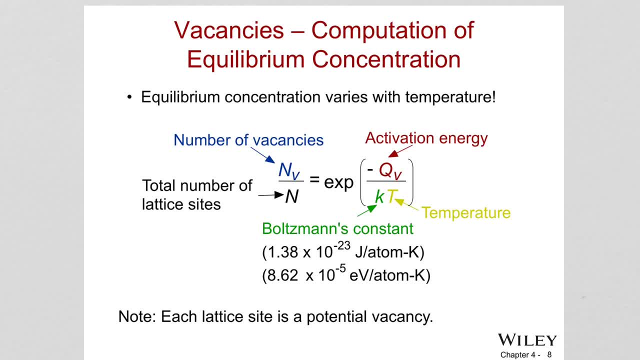 it actually lowers the overall energy of the structure. so by thermodynamically, structures need to have vacancies. so there is no way there could be a perfect arrangement because there will always be vacancies. and and then how do we know the equilibrium concentration of vacancies? equilibrium concentration means: 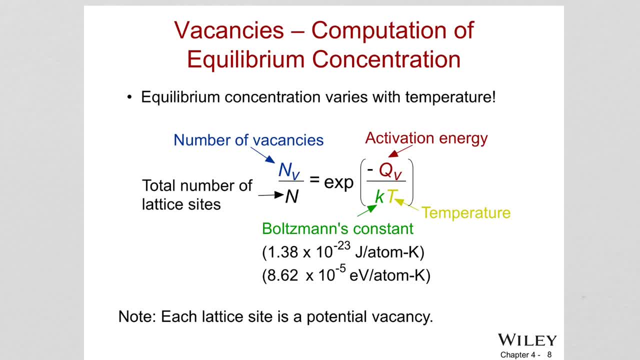 thermodynamically equilibrium, right. so systems always reach thermodynamic equilibrium. and at that temperature, at that position, what is the equilibrium composition of the vacancies in the structure? what, how many number of vacancies you should expect at that temperature? of course it also tells you with temperature equilibrium concentration of the vacancies are changing. 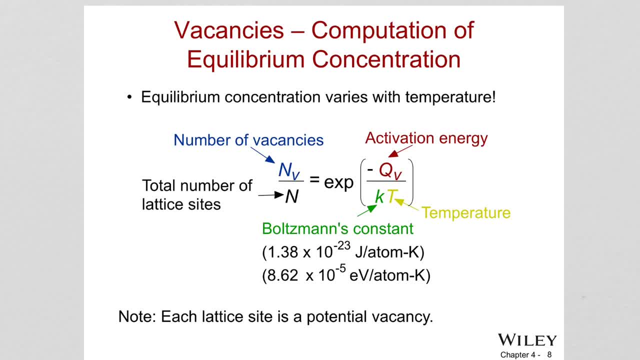 okay, with different structures, there will be different amount. with different temperatures, there will be different amounts of vacancies in the structure. so how do we calculate the equilibrium concentration? and we are given this equation: and n the capital. n is the total number of atomic sites, q is the activation energy necessary for the formation of a vacancy. 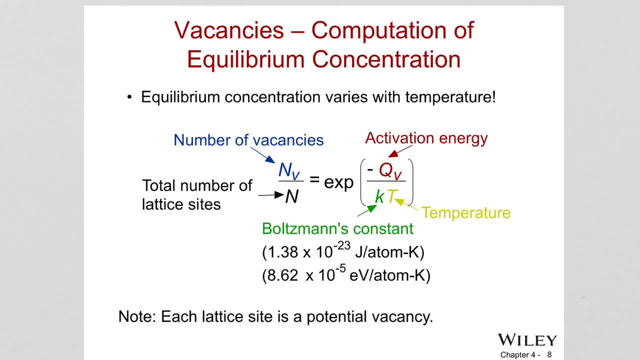 k is the Boltzmann constant. with different units it can be given depending on what type of energy, what type of units the activation energy is, and t, of course, the temperature. and what we are trying to figure out is n with a subscript. v is giving us the number of vacancies. 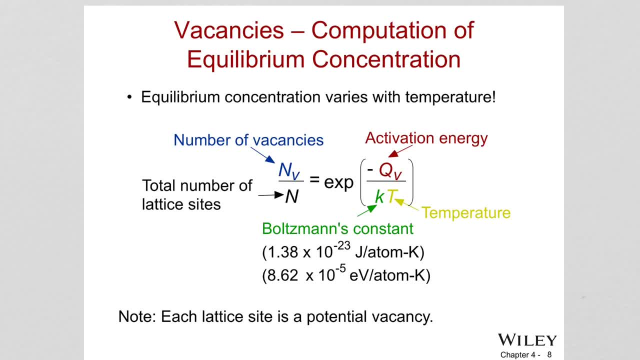 and what we are trying to figure out is n with a subscript v is giving us the number of vacancies, which is equilibrium concentration of vacancies at that temperature and of course each lattice side can be can be form a vacancy. each lattice side can form a vacancy- e, and the number of vacancies they are going to increase exponentially with temperature. 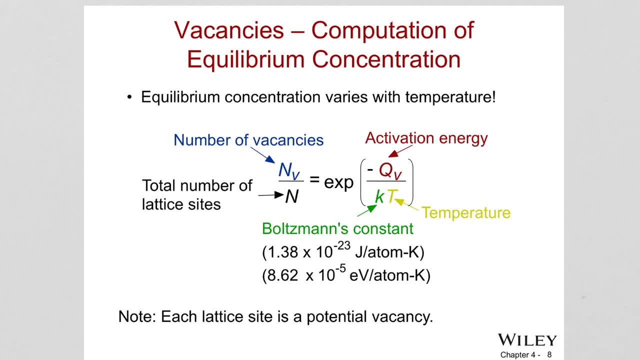 so one way, one example, if there are. this ratio is usually is around ten to the power, minus four for metals below their melting temperature. so that means one lattice side out of ten thousand of four is going to be room temperature minus four metal inside the inflating ice. geschrieben on paper. 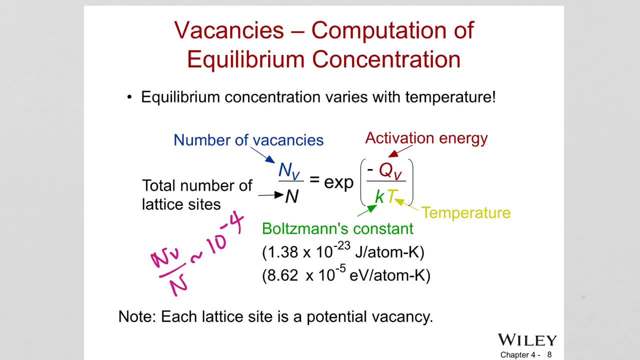 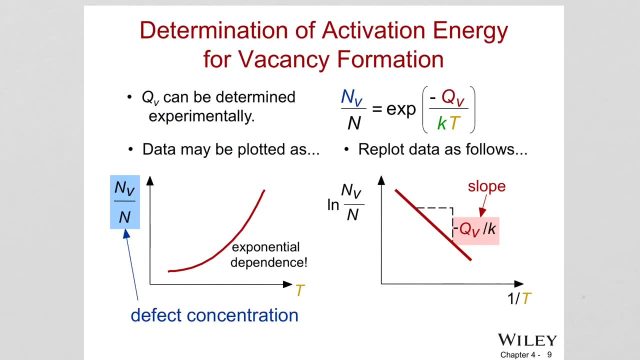 will be empty and it can be any place. okay, there can, it can be in any place. so how this activation energy can be found? usually, experimentally, we can find activation energy. normally, if we want to plot this equation, it will do show you an exponential dependence. right, assume this is the Y, okay, and but if you take 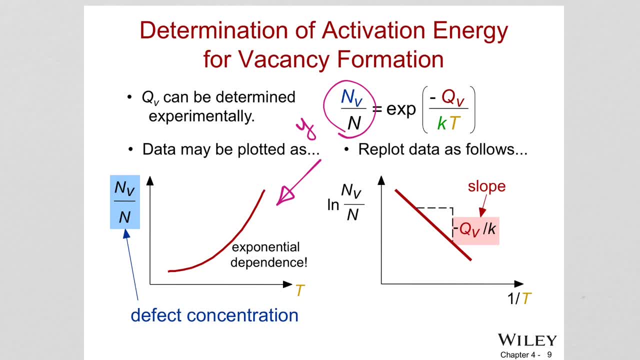 the logarithm of both sides. you will see it's actually a line equation and the slope, if you plot this one against 1 over T in the line equation, taking the logarithm of both sides, and then it will give you the slope, will give you the 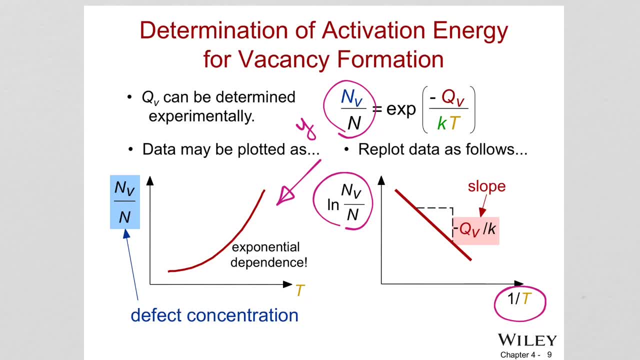 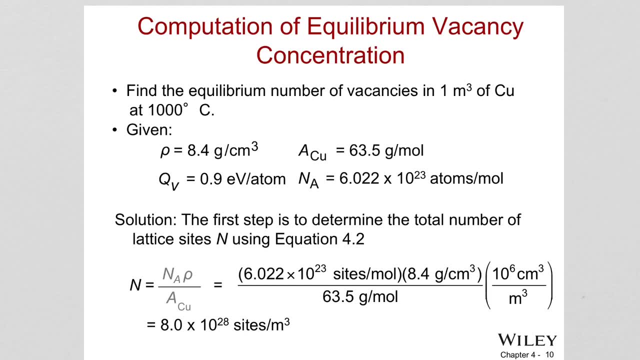 activation energy. K is the Bolton constant, remember that's a constant. so one example is given to us compute the equilibrium vacancy concentration for copper. that is at 1000 degrees C. so always needs to give the temperature because it depends on the temperature in one meter cubed. 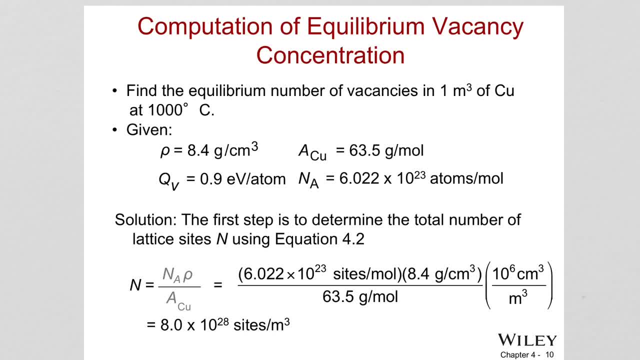 one meter per cube of copper at 1000 degrees C. so the first thing we need to figure out the number of atomic sites per cubic meter for copper. and here is the equation for that. let's understand it. so I know. in one mole there is a. 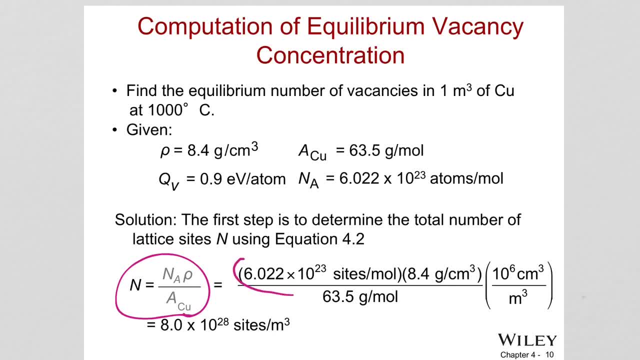 mole, there are a vagina, number of sites attempts right, and one mole is this much gram. so 6.022 times 10 to the power of 23 Adams is actually 63.5 grams. okay, and but what is the density? density means what is the gram in a in a centimeter cube. so one centimeter cube is eight point four grams. 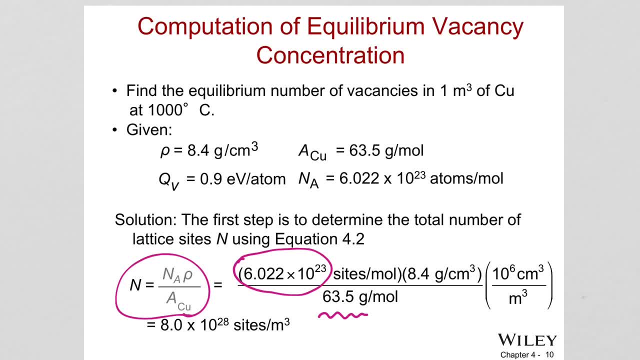 so this will tell you then, how many numbers of atoms are there. atomic positions are there in one centimeter cube, and you can also look at the units to understand that right so, one mole. there are this much of atomic positions, but we don't have one more. we want a one centimeter cube of. 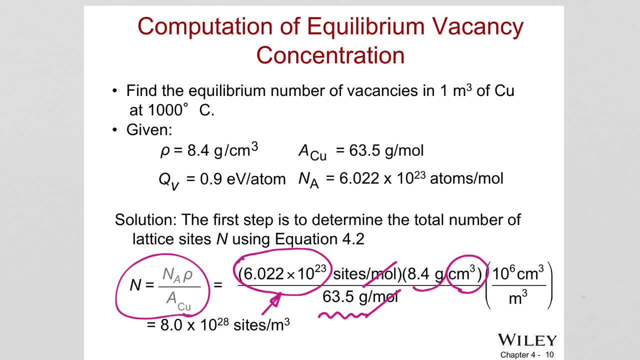 okay, and one centimeter cube of it is this much gram compared to that, okay. so what happens here? you are gone, grams are gone and centimeter cube is converted to meter cube. it tells you how many sites there are at the end in one meter cube. and we already have one meter cube, so that 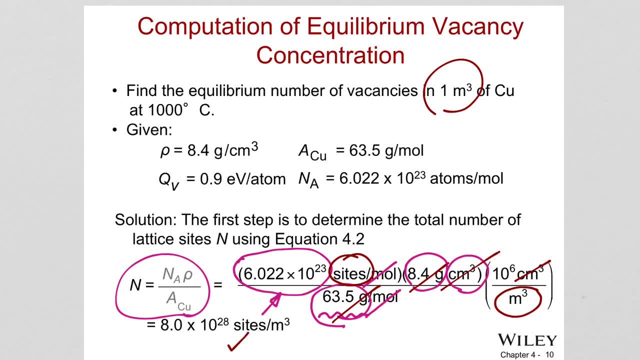 is okay. so this much sites in one meter cube. so density is given you, giving you what is the mass in one centimeter cube, or meter cube, right in volume, what is the mass in one unit volume? and we, we also know how many sites are there in one mole and what is the mass of one mole. 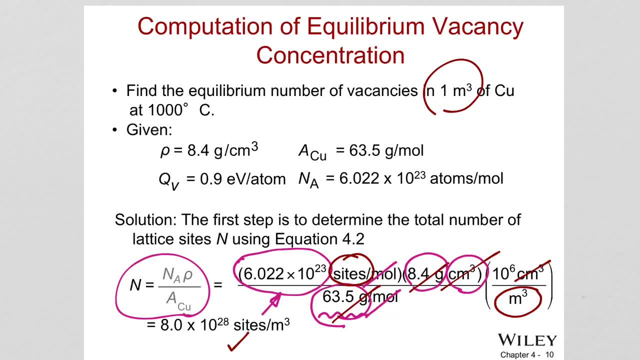 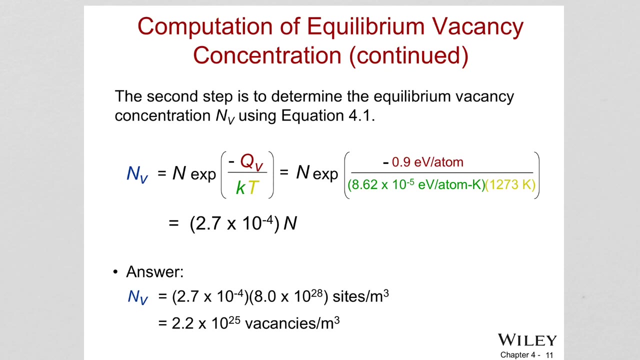 but what we are doing is we are trying to convert it. in a way we can see how many sites in a volume. so therefore we do it this way and then, therefore, we calculated atomic sites in a unit volume. once we do that, and now we can plug it into our vacancy equation, which will give us the equilibrium. 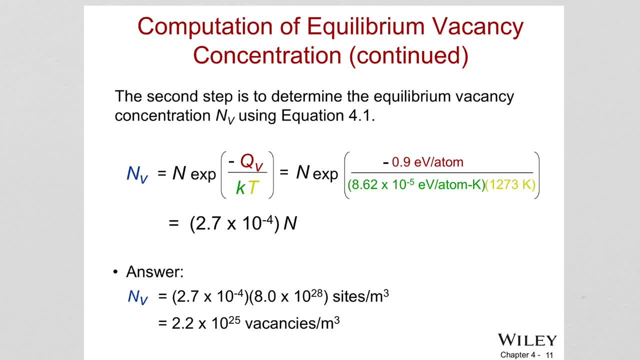 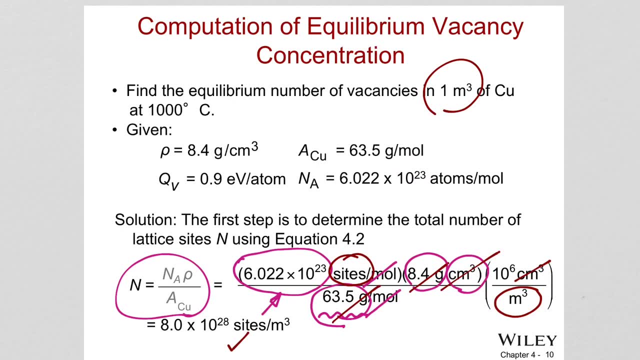 vacancy concentration at that temperature and of course some things need to be given in this equation. so you figure out n, you figure out the mass of the atom and you can see that the mass of the atom is equal to the mass of the importa. exemplify that we are created in our body: droid mass. 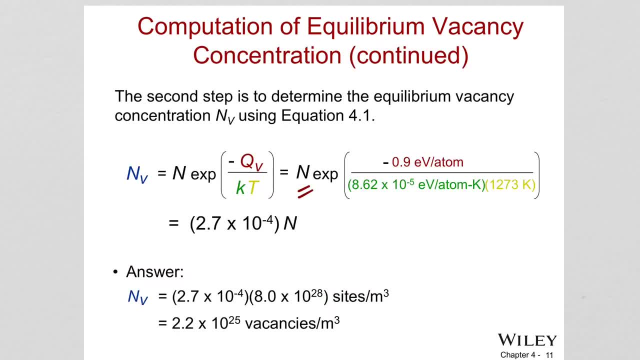 quatern, To say, is equal to the mass of the n us, in other words, is the mass of the atom, and so e to the amount of mass in it, based on the crucible mass of the happens all in order that we have. the Ant Eb times line will deactivate all of these Columns. will also be in K. 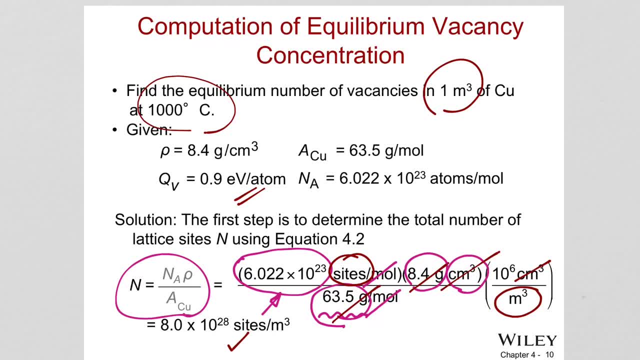 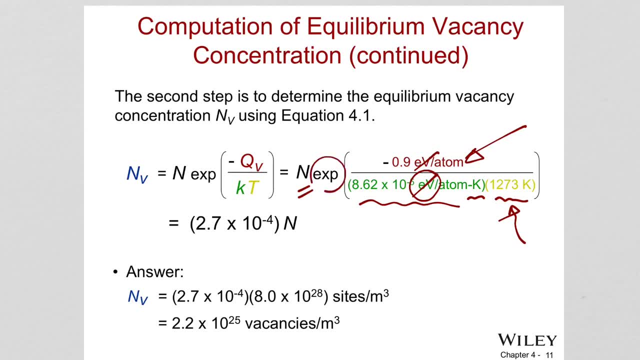 meet m the gently y can choose what we'll see. also, yeah, before starting the example plus high 1999 Is to take check states and our next step, so you're gonna put in the Kelvin- and don't forget, this is exponential right- and then, if you do that, you will figure out basically the answer. the answer is: 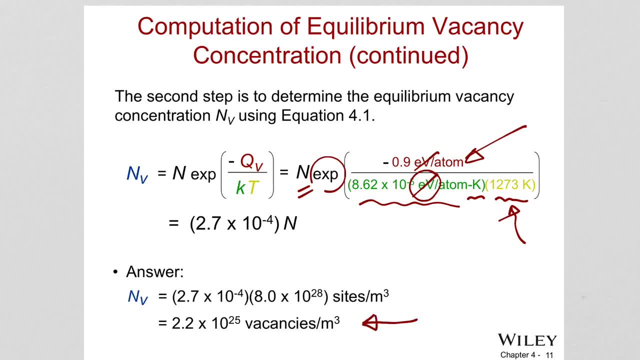 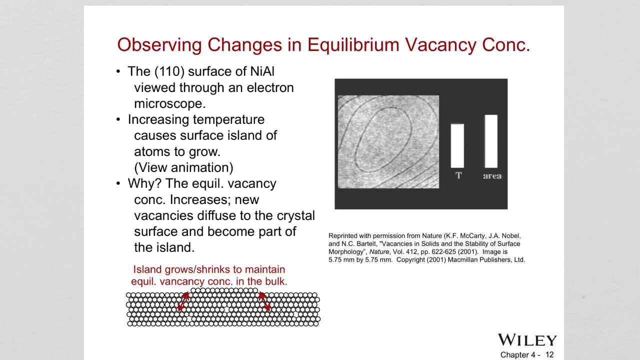 this much weight equilibrium vacancies in one meter cube of that material. so each meter cube of copper, you need to have this much of vacancy because that is what thermodynamics says. okay, okay, so this is taken from a study. we cannot see the video and I couldn't. 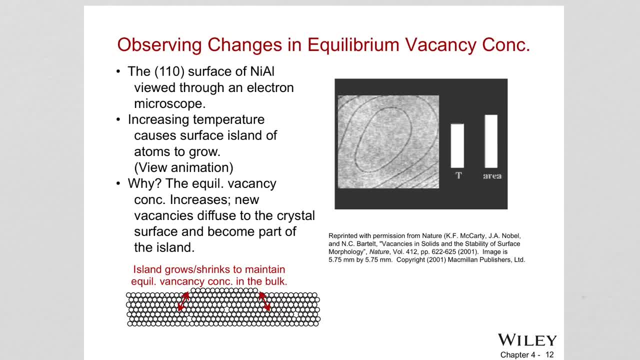 locate it online. but we are seeing a microscopic image with an electron microscope. it means in very small scales. okay, there is a material, it is certain. face her face of it. we are seeing how the islands form while islands form the reason. yes, they are changing the temperature during the 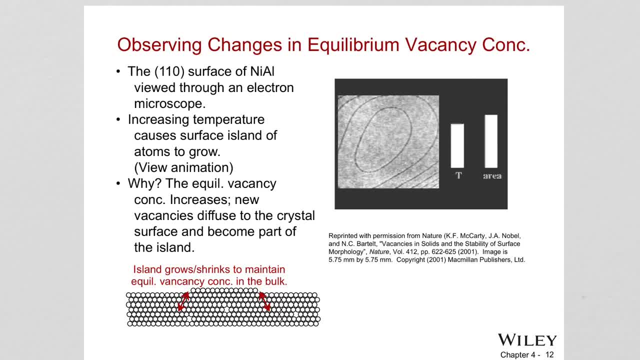 recording. so this is like a liar recording. they just change the temperature and also monitor it under microscope. okay, so what happens is that when they change the temperature, the equilibrium cool, vacancy concentration also changes, right? so if we increase the temperature with more vacancies have to form thermodynamically. 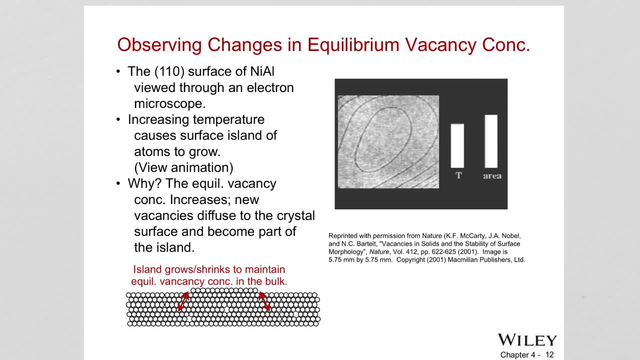 in the structure. of course, the formation of new vacancies will push the atoms forward, like forming, like islands, like that right, so it is pushing the. the vacancies are forming, push, atoms are pushed and it is like islands are forming and that's what they are seeing under the microscope. they are seeing these regions as black lines here. okay, so like 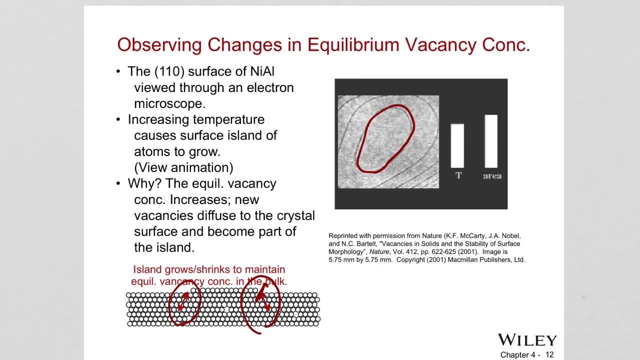 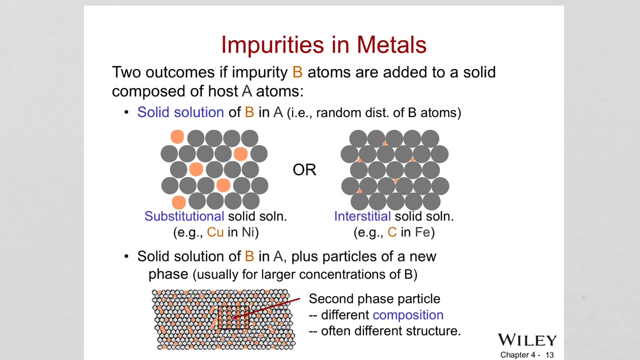 the atoms are pushed forward and then because the material, bulk material inside has to accommodate for more vacancies, that's it. so it just tells you that by increasing the temperature you are also changing the number of vacancies inside the material. So having a pure metal like 100% the same atom, this is just not possible There. 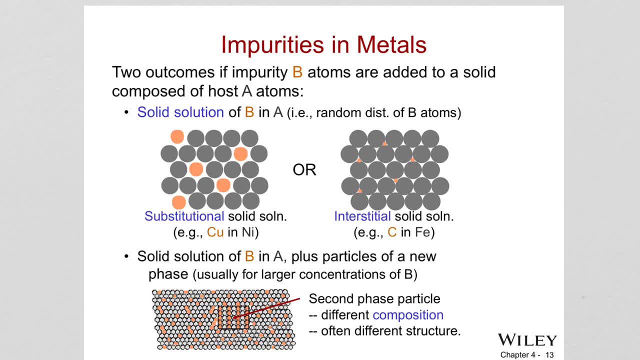 will always be some impurities, some foreign atoms that will present And of course we call these defects in the structure. but, as I said, they can be positive and negative effects of these impurities. And we have actually seen that in chapter 1 where I discussed how 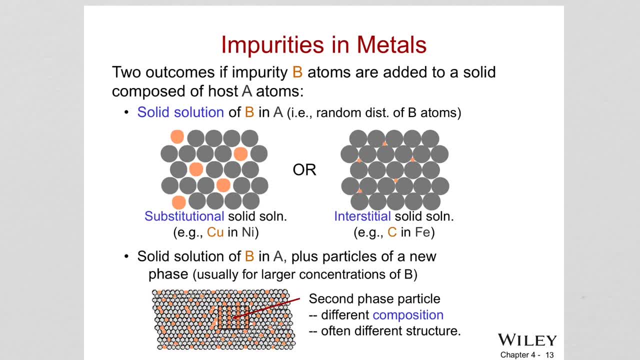 addition of certain elements, such as adding nickel as an impurity to copper, changes the electrical conductivity. So you can manipulate the conductivity with the addition of nickel to the copper. In that case nickel is called impurity, But it's just another type of atom. 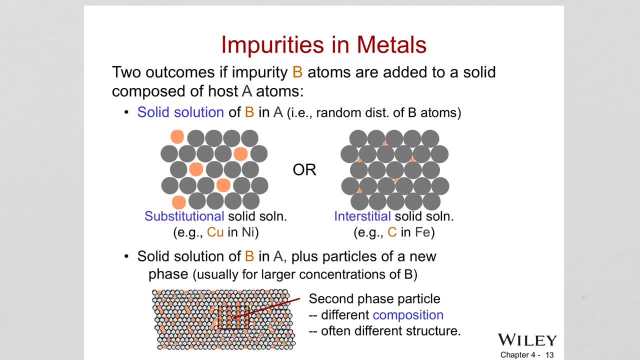 that you are adding to the copper matrix, copper structure. So in this case we have two outcomes, Like if the impurity is B atoms and the hosts are A atoms, adding B into A, just like adding A into A, is not possible. And if the impurity is B atoms and the hosts are, 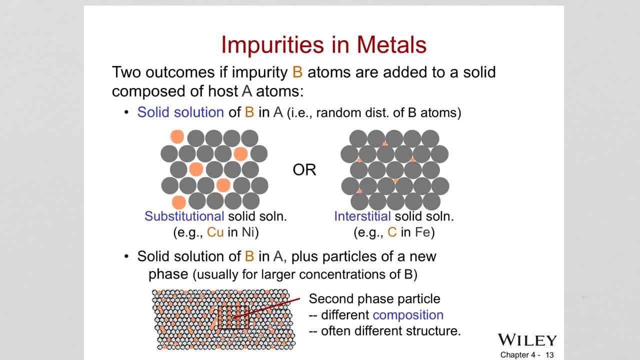 nickel into copper. nickel is b and copper is a. at that time two outcomes, two way right. and let's see, of course they give another example here, the same. but then they said: nickel is the matrix, they add copper, that's also fine, that's fine. both ways can happen. and so one outcome is: 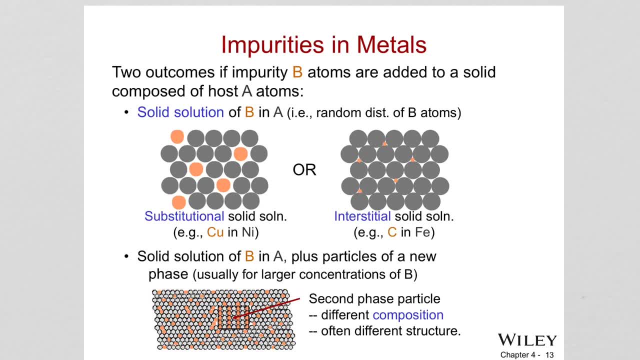 forming solid solution. okay, and what is a solid solution? so, when you have a solution, think about you have a solute and solvent, right, one needs to dissolve in the another, like think about you are dissolving sugar in water. sugar is your solute and the solvent is your water. 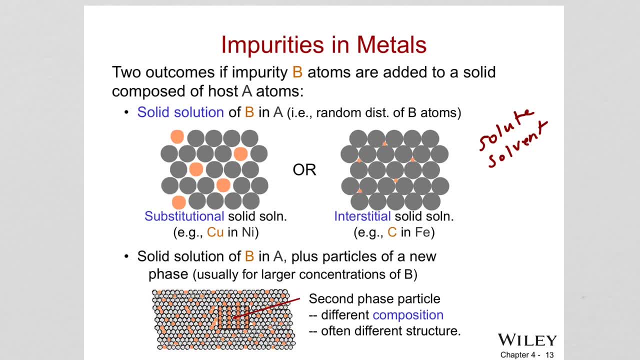 okay, right, solvent here is the element or the compound that is present in greatest amount. it is like they are- you can call them host atoms- and the solute is an element or a compound that is present in minor concentration. in this case, the gray ones are the host. 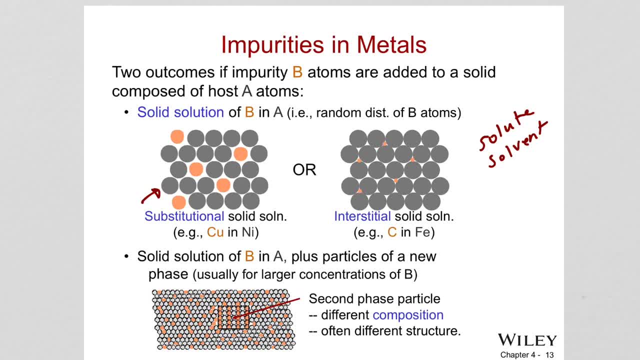 a solvent and the orange ones, the b, is the solute which is in minor concentration. so solid solution, as we said, can have two outcomes. okay, if we mix atom a and b it can be a substitutional solid solution, meaning just regular lattice sites in the solvent a. 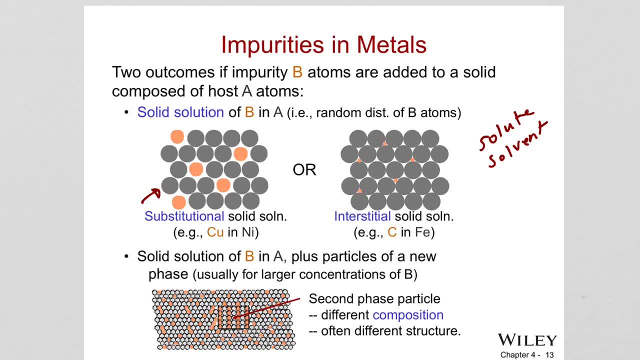 regradingatz, regular lattice sites are just replaced with solute B atoms. so in this case, regular nickel atom sites are exchanged with copper atoms. okay, and another way this can happen: if we mix A and B and form a solid solution. another way this can happen is interstitial solid solutions. this is 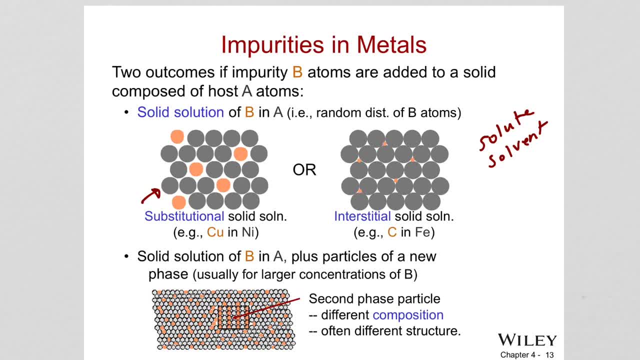 where we call it copper in iron. usually one of the examples- and these are also called alloys, right alloys, addition of minor amount of elements to a matrix of another element. in this case we have the major component- is the base, is the solvent, is the iron, and when the iron packs atoms in the 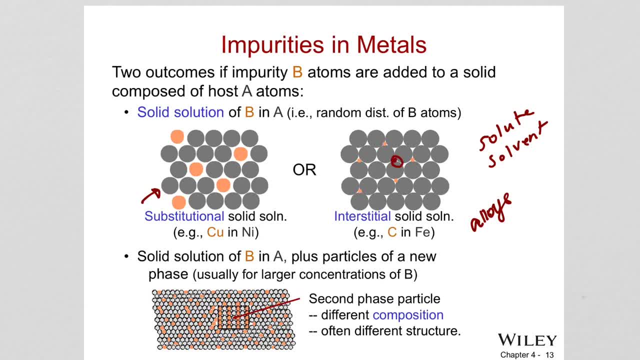 in these atoms there are empty regions, like this one right, and those are small, can accommodate small elements, small atoms like carbon. so carbon can fit into those interstitial sites in the, in the packing structure of iron, and this is what we called interstitial solid solutions. so two type of solid. 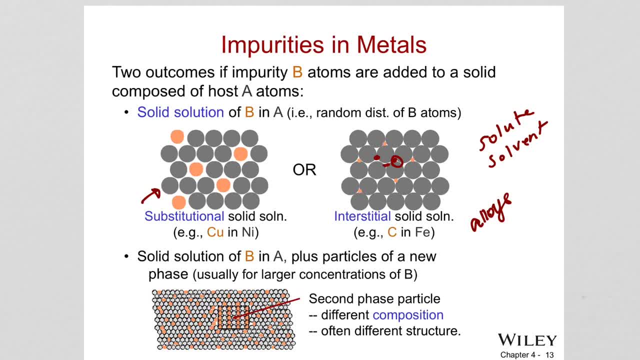 solutions is substitutional and interstitial solid solutions. we need to understand something very important here: when we have a solid solution, this is just one phase, meaning everywhere the structure is the same everywhere. So copper is dissolving in nickel, in this case right, It's forming a homogeneous structure by itself. There can also be second phase particles, another phase which has a different composition, which has a different structure. 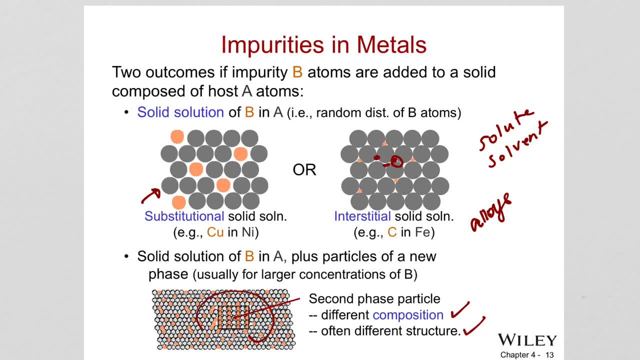 So, overall, if you look at everywhere around here, right, This place, this place, that place, they are all having a solid solution. Copper is dissolving in nickel, But at certain regions they are actually reacting only at certain ratios, like this, within the square. you are seeing, right. 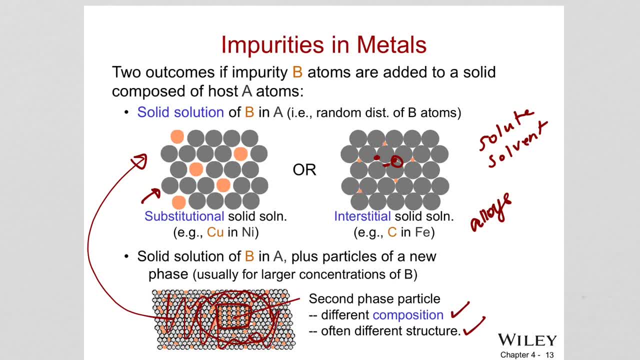 They are actually forming some type of a compound, maybe copper, nickel compound or something. So they are actually the composition. The composition is different there, The structure is different there. Therefore properties are different there. So within that solid solution there can be new phases, And we call them second phase particles, And they can have different composition and different structure. 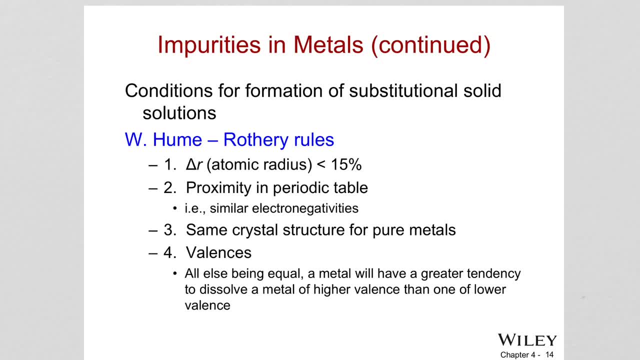 So several features of the solute and the solvent atom. The solute and the solvent atom determine the degree to which the former dissolves in the latter. So basically how much they dissolve in each other, And there are certain rules for that. Okay, They might be completely dissolving in each other. 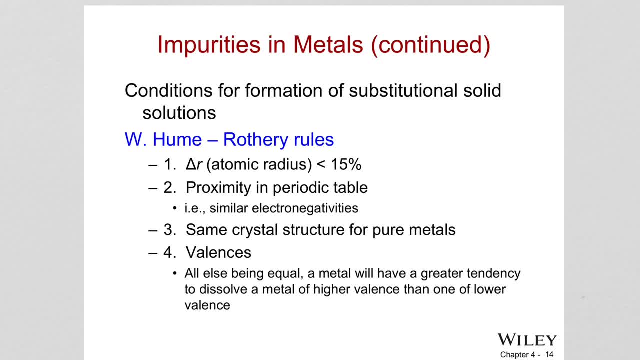 Let's say you put a little bit of salt in water and you cannot see the salt anymore. right, It is totally dissolved. But let's say you put sugar in water, You keep putting, putting, putting And at some point it cannot dissolve in it anymore. So there is a limit, right? 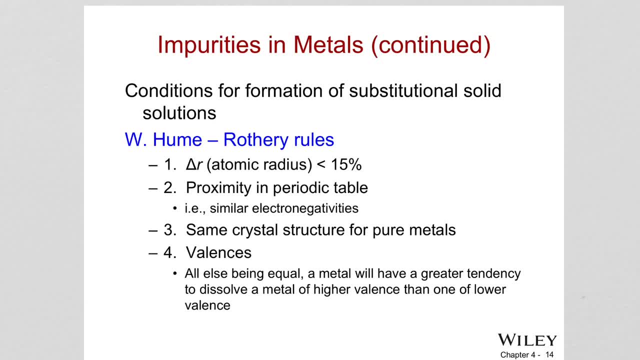 So what are the things that are determining how much they dissolve in each other? And this is determined by a scientist, a material scientist, Hume Rodri, And he developed certain rules to understand, To understand How much, basically, two atoms are capable of dissolving in each other. 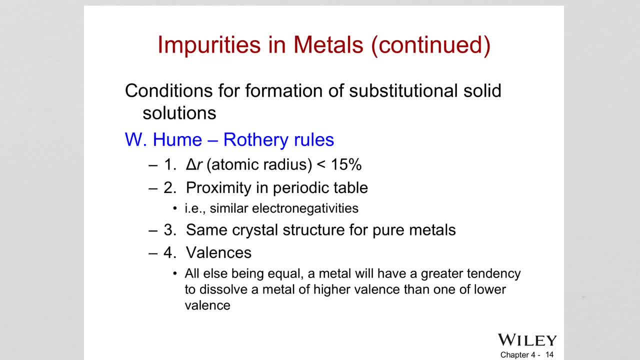 So the first one is atomic size factor. Of course let's say copper and nickel, right? We need to look at the sizes of each of these atoms In copper and nickel. copper atom size is very close to the nickel atom size. 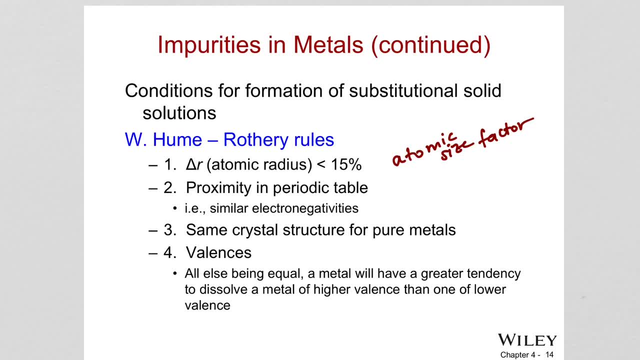 So they are very easily dissolved in each other. So what we are looking at as a rule, if we want appreciable quantities of a solute to be accommodated in the solid solution when the difference in atomic radius between the two atoms is less than about 15%. 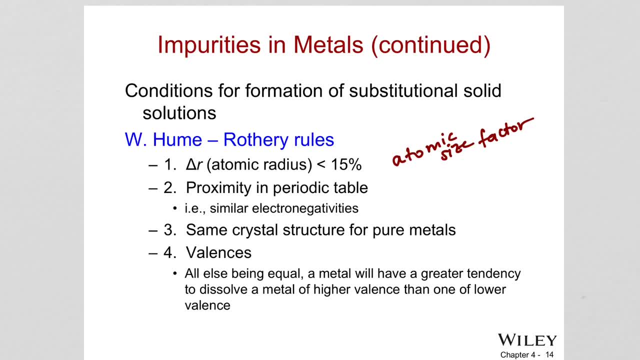 So let's say nickel and copper, the atomic radius difference is going to be, should be less than 15%, to be these two different atoms to dissolve into each other, To take the crystal structure of each other. So the second is: the second is electronegativity factor. 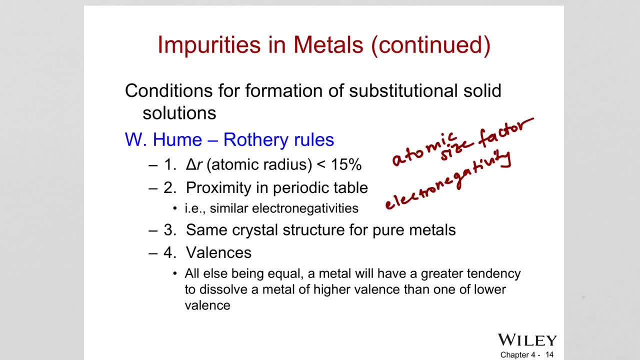 So two atoms. if they're going to form appreciable solubility in each other, their electronegativity should be close to each other, Because if their electronegativity is not similar, then they will react to each other And this is going to give us a compound. 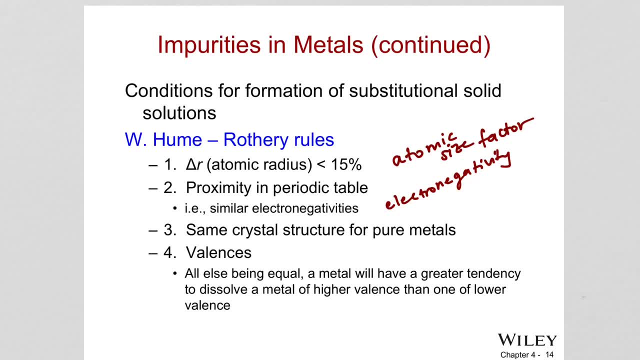 a reaction at certain ratios. a compound like the compound is like silicon nitride. right, We don't want this compound because the solid solution is basically atoms replacing the other atoms place or interstitial places, So basically electronegativities should be similar. 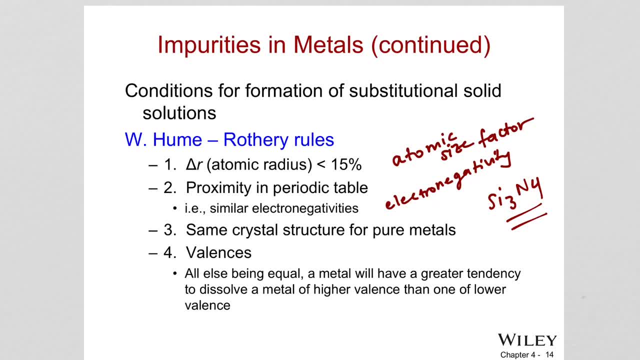 should be similar for appreciable amount of solubility in between each other. okay, So the next thing is same crystal structure for pure metals. So if one, let's say, has FCC like nickel, another one should have FCC to support this solubility in each other. 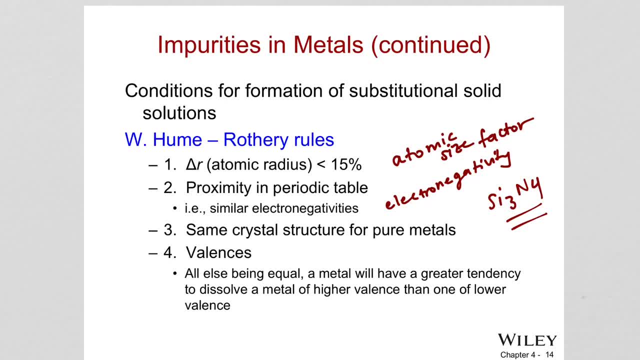 because then it is easier for atoms to take place of the another host atom, right Impurity to take place of the host atom If both has the same crystal structures, they are both FCCs, they are both BCCs, etc. 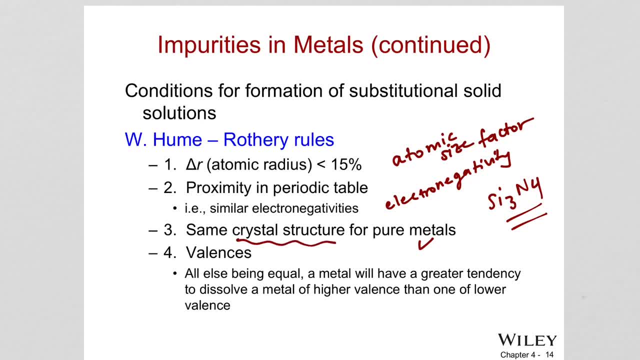 Okay, so crystal structure. And the last one is valence. So this is interesting observation. What happens here is a metal has more of a tendency to dissolve another metal of higher valency than to dissolve one with a lower valency, So number of valence electrons are affecting these. 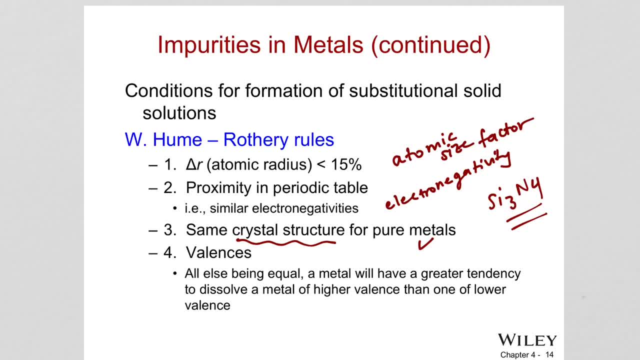 So if you have a metal, it has a more tendency to dissolve another metal if it has higher valency, higher number of valence electrons. This is just observation, okay. Best example to this is always copper-nickel solid solution. Their atomic radius are very close. 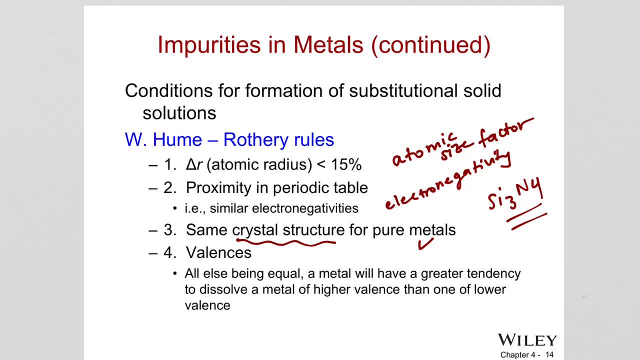 One is 0.128,, one is 0.3.. One is 0.125.. They both have FCCs and their electronic activities are. one of them is 1.9, one of them is 1.8.. So 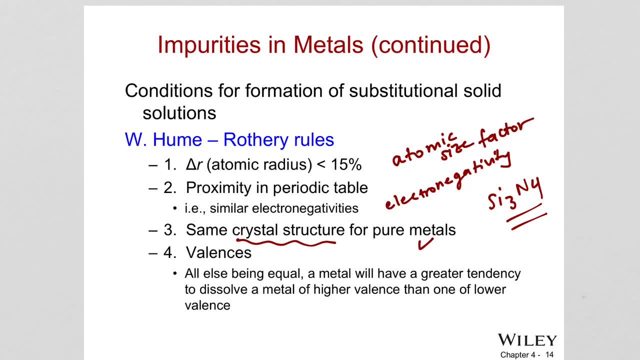 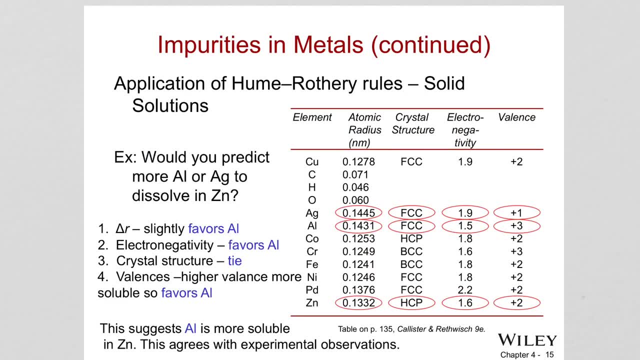 therefore, it is very easy for them to form a solid solution basically. So let's look at it. So something like this can come right, Given the table like the picture here. So would you predict more aluminum or silver? 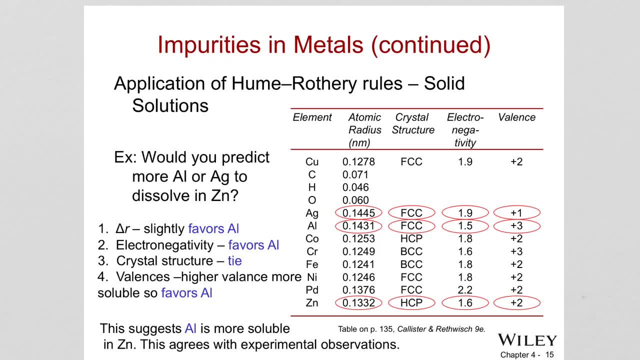 to dissolve in zinc. So first we need to compare atomic radius. So we are looking at the zinc and we are looking at the atomic radius of silver and aluminum. which is more closer to zinc. okay, The one, aluminum, is more closer to zinc. 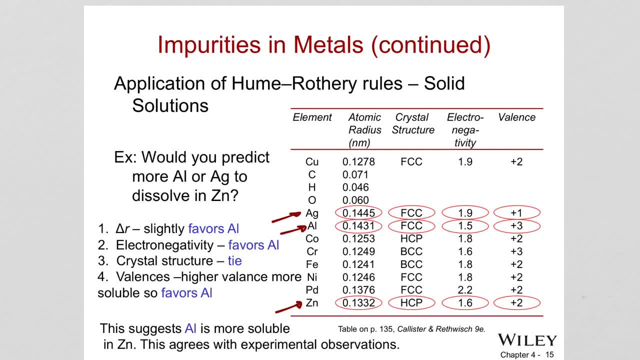 Of course both are different, not exactly the same, But aluminum is closer to zinc. What about electronegativity? So one is 1.6, aluminum 1.5, silver 1.9.. So 1.5 is closer to 1.6, right. 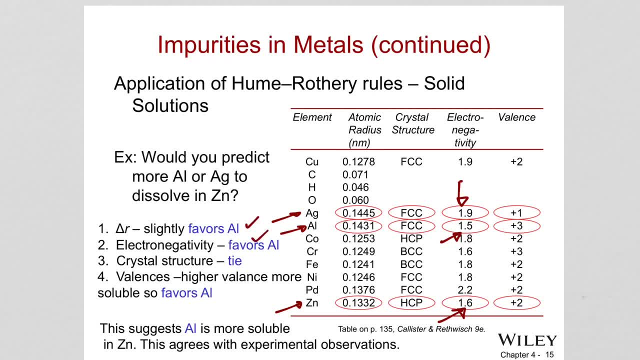 So again, it favors aluminum. When we look at crystal structure, this is hexagonal packed but it's a closed packed structure And this structure is similar to FCC also. okay, So HCP is also most FCC and HCP most dense packed structure. 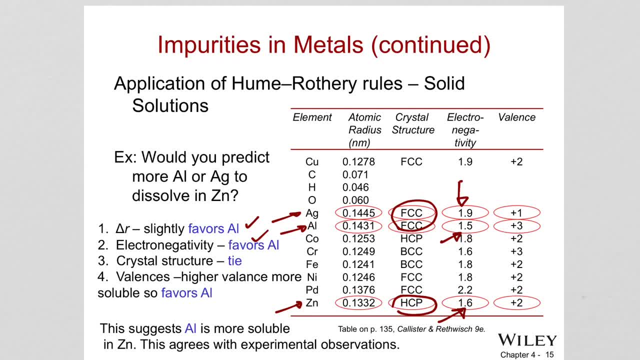 Remember, coordination numbers are the same right, So those structures are similar. Both are FCC, So there is no difference in terms of aluminum or silver that can dissolve in zinc, So that's a tie, And which has higher valence. 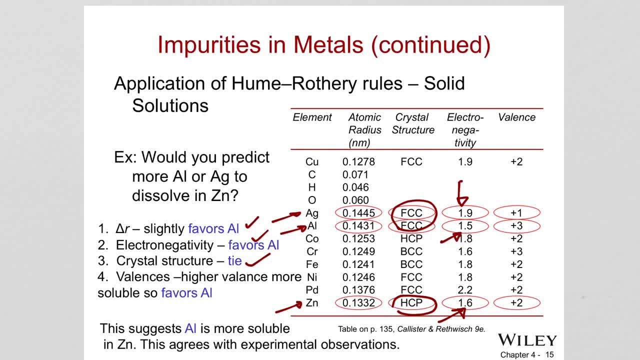 Because that will be the favorite. So this is plus 2.. We want something bigger than this. And plus 3 is aluminum. Okay, so aluminum is favored compared to silver, So this suggests that aluminum is more soluble in zinc. 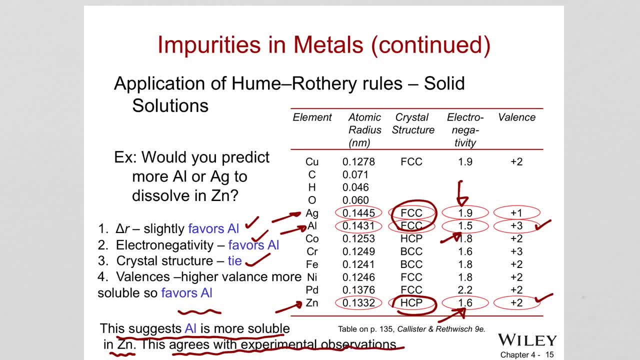 And this agrees with experimental observations. Okay, so these are some rules. people come up based on observations and based on some theoretical calculations And we are seeing that atomic radius difference, crystal structure, electron degree, negativity difference, valence, electron difference, those are affecting the solubility. 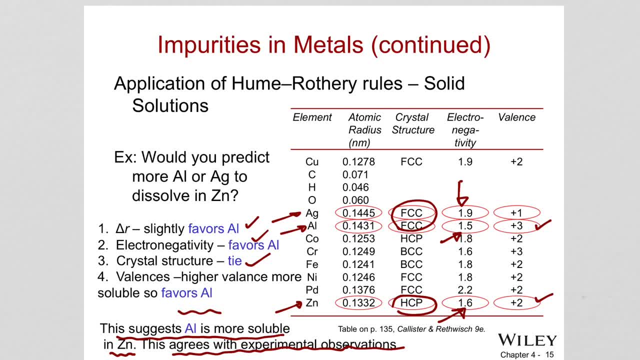 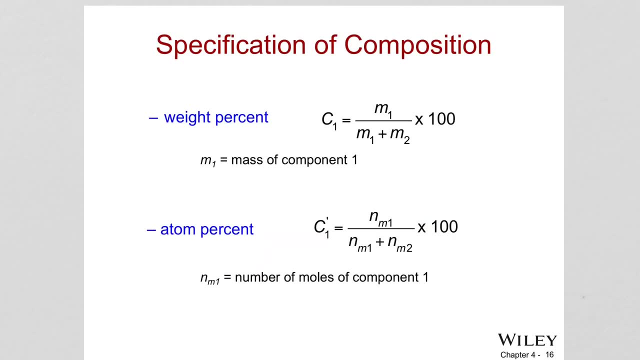 And from tables as such, we can predict. we can predict. of course, we need to confirm it with the experimental observations also. Just one thing to understand: When we say solid solution, okay, that is a single phase, mixed perfectly, Okay. 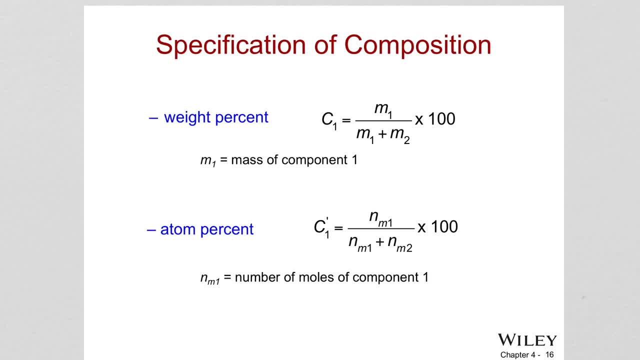 but when we say alloy, alloy can consist of one or more solid solutions, One or more two phases, And they can have different crystals, different crystal structure, with different chemical compositions. Okay, So when we are trying to specify the composition of an alloy, 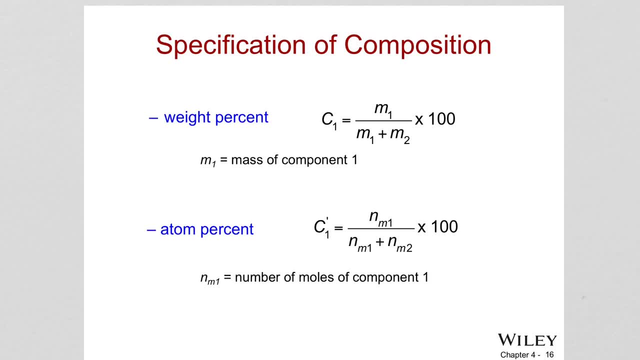 we can specify two ways. We can specify the composition as weight percentage or atom percentage. Okay, For weight percent, of course it is going to be the weight of a particular element relative to the total alloy weight. So in this equation, 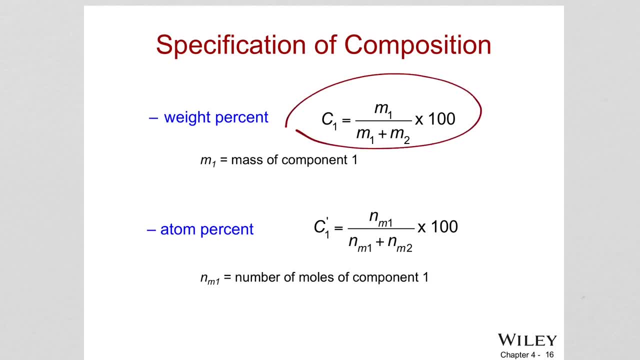 we are seeing here right. So m1 and m2 basically represent the weight or mass of elements 1 and 2 respectively And this will calculate basically the concentration of atom 1.. And if you change m1 in the numerator with m2,, 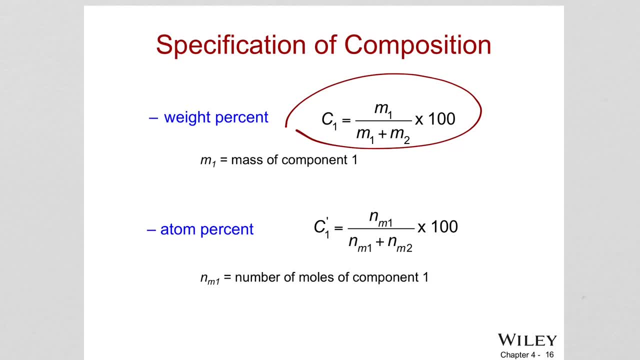 of course, it is going to give you the weight percent of atom m2.. The atom percent is calculated by this equation. here we are seeing. What is that? That is basically the number of moles of an element in relation to the total moles. 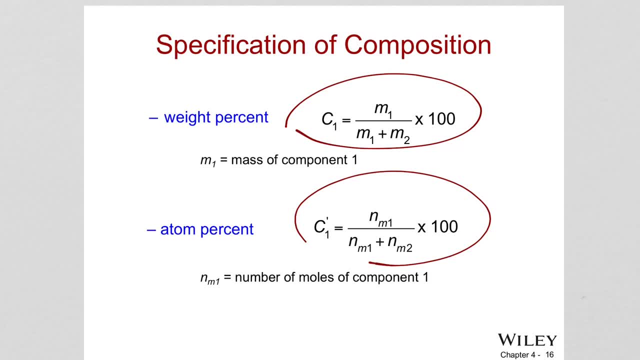 of the elements in the alloy. Of course, when you change m1 with m2, n1 and m1 with m2, this will give you the atom percent of the second element In this equation. just, we are calculating the atom percent. 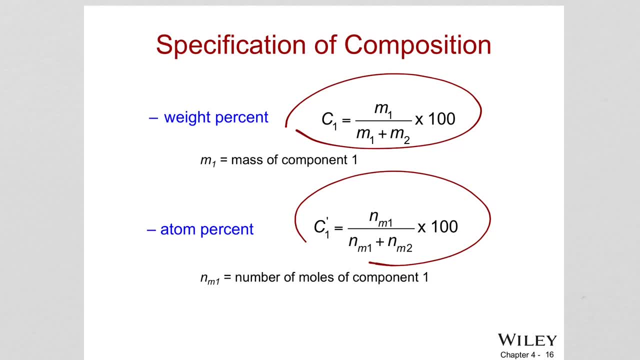 of the first element, element 1.. Okay, All you have to do is find the number of moles of component 1 and divide it to the total number of moles in the overall material And, of course, multiply these both equations with 100%. 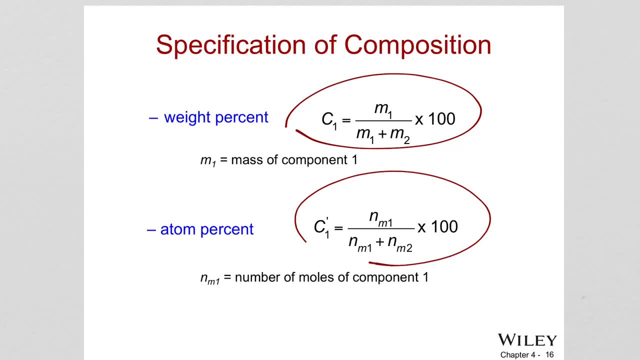 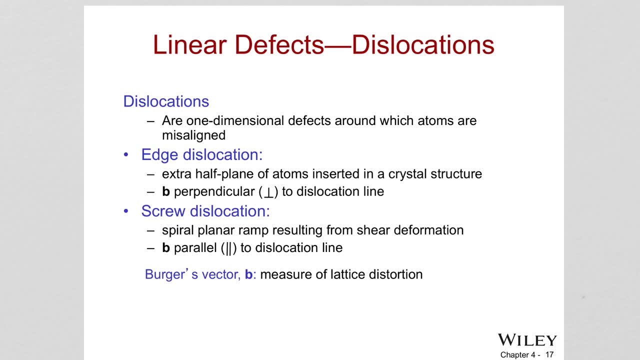 So we can talk about percent weight, atom weight percent or atom percent. So the first ones were point defects. we learned, And now we're going to learn about linear defects, And this defect is so so much important. Okay, This is dislocations. 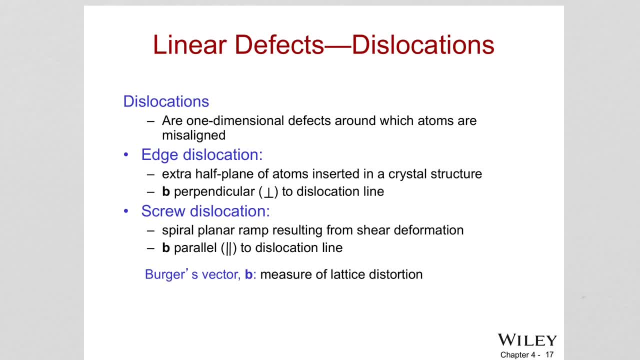 Another name. So linear defects are also called dislocations. Okay, These are one-dimensional line defects. Along a line, the atoms are misaligned. This is not a single atomic point. Okay, Where there is zero dimension, This is one dimension. 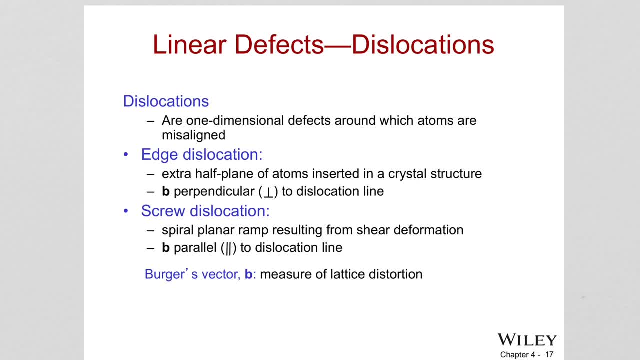 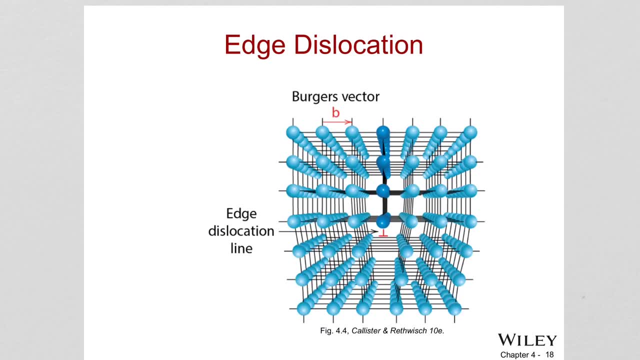 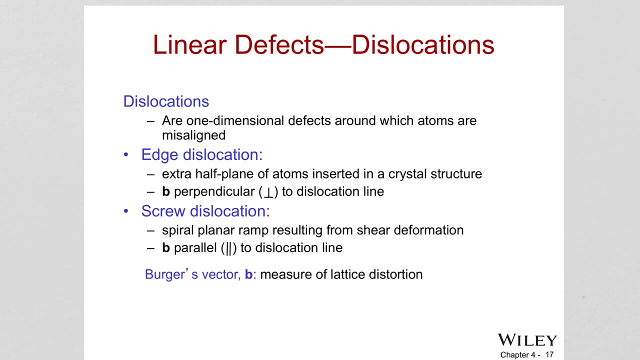 There is a longer line, Okay, Along the line atoms are misaligned. So these are dislocations. So there are two types, Okay, One is edge dislocation And this is, you can imagine, like an extra half plane of atoms. 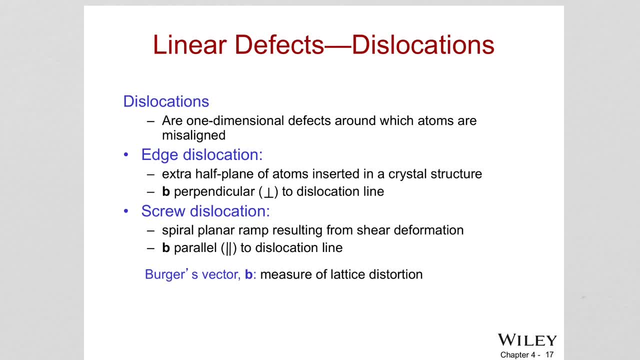 are inserted in the crystal structure, creating disorder, And B is what we're going to call the Burgers vector. Let me write it. It is a vector that we're going to use to talk about magnitude and direction of the lattice distortion associated with. 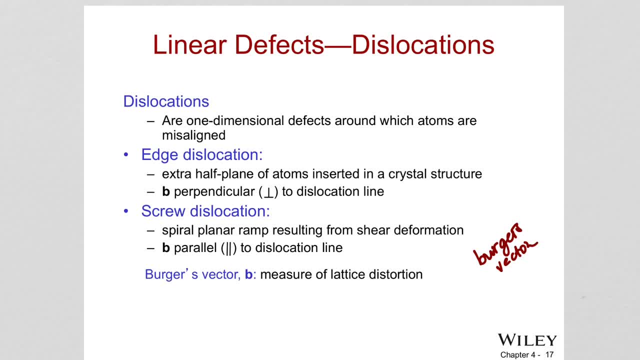 the dislocations. So let's just for now, let's learn. edge dislocations are extra half plane of atoms inserted in the structure And we are showing it as this with this symbol like upside down T, This part here representing extra plane. 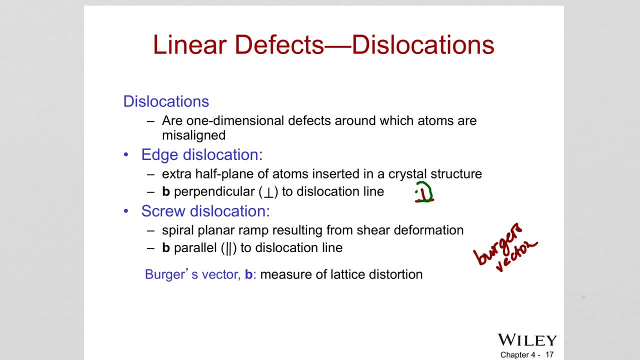 of atoms being inserted into the lattice, And this part is that plane. Okay, That plane, that extra plane of atoms sit on, Okay. So next is screw dislocations- Spiral planar ramp resulting from shear deformation, And in this case, 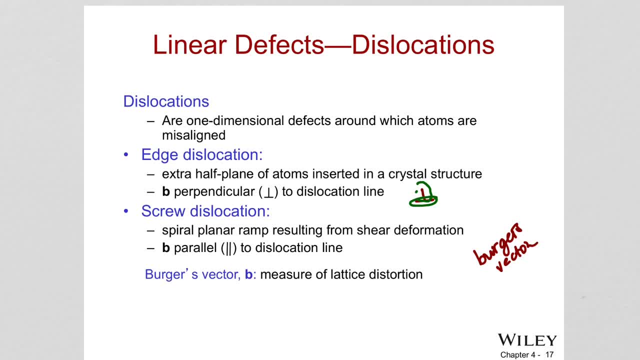 Burgers vector will be parallel to the dislocation line. In edge dislocation, Burgers vector is perpendicular to dislocation line. Okay, So we all gonna see what that means. Okay, So Burgers vector is a vector we are using. 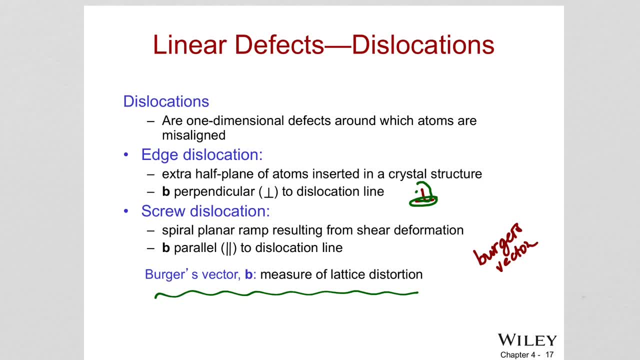 to describe the magnitude and direction of that distortion in the structure. Basically, this is due to the presence of dislocations. So let's start with understanding what edge dislocations are. So understanding dislocations requires a little bit imagination, And I send 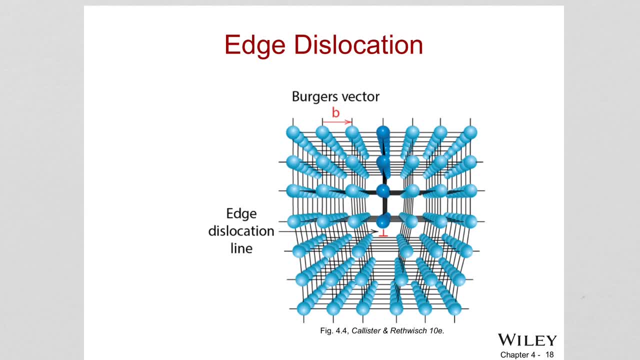 you guys some animations, But try to check all the images online and try to see if you can grab the visualization of the object in your mind. Okay, In this case we are seeing the edge dislocation, Which is these are the normal. 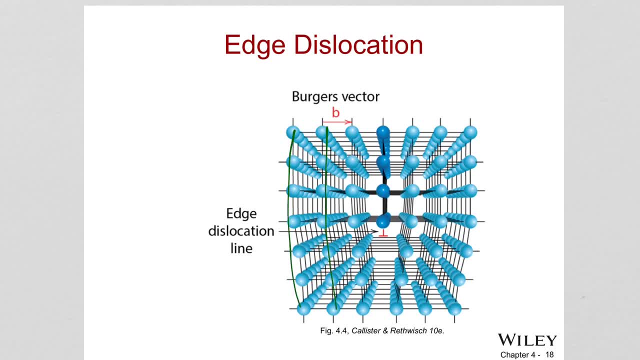 lattice atoms. The atoms sit in their perfect order, But what happens here? a half extra half plane of atoms is fitted into the structure, Okay, So of course it is shown with, as you can see, a upside-down. 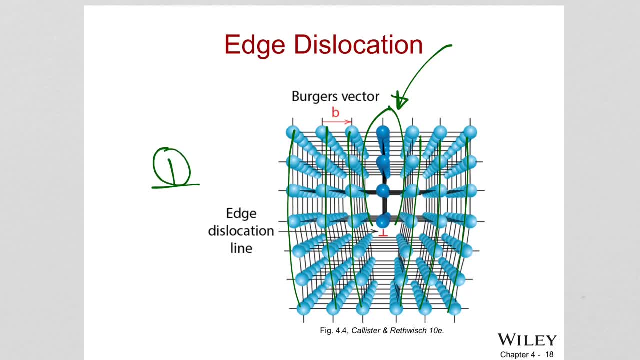 T, This part representing the extra half plane that is inserted into the perfect lattice, And this is where the, this is the plane, basically This plane, that where that extra half plane of atoms sits. Okay, So where does dislocation or line? 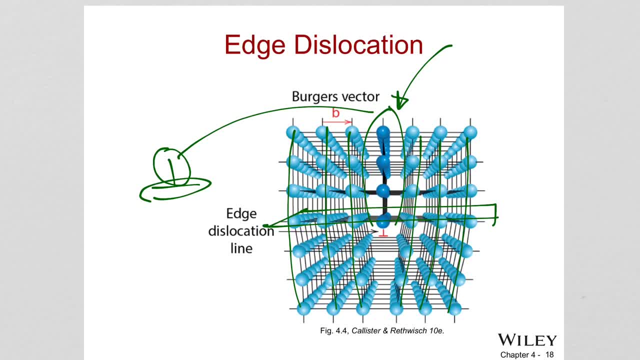 term conforms. where does distortion happens? The line is: you need to look at to the through the screen. So in 3D, we are going into the screen. We are going into the screen. Okay, So here. 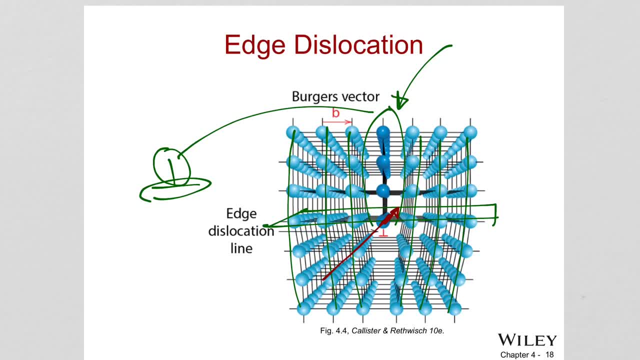 this is the line. Okay, The atoms sit. We are going into the screen. All these atoms. they are sitting on the dislocation line. So what we are seeing is what we are seeing right there. let me do this. 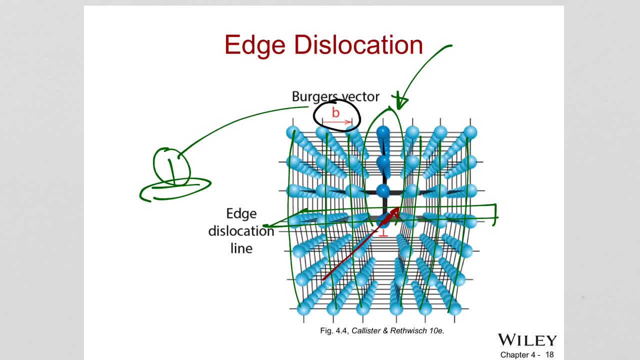 what we are seeing right there is showing us the direction and magnitude of the lattice distortion. Of course, with the addition of this extra half plane atoms, our lattice is distorted Right. Every atom move out of their place because of this dislocation. 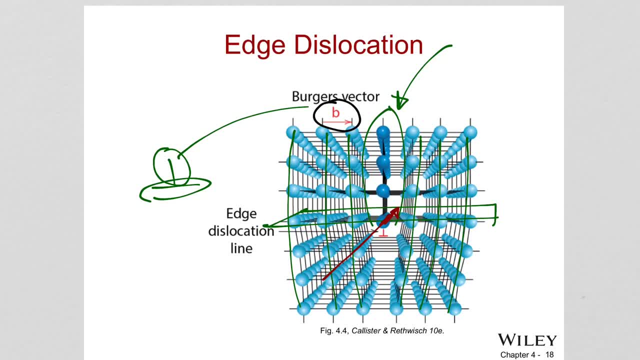 defect. So there is some distortion in the lattice. But how much And what's the magnitude? Right, Those are shown with the Burgers vector B. So to understand that, let's walk in unit 3.. 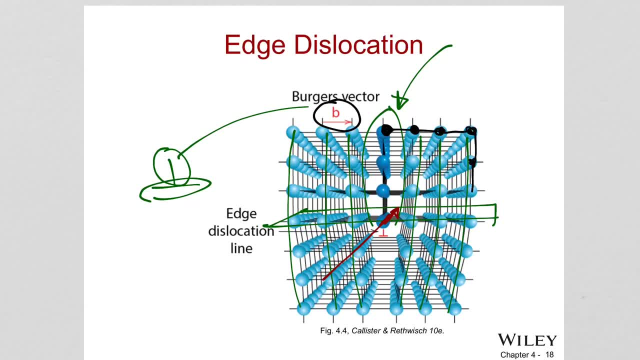 I move here Down 1,, 2,, 3,, 4,, 5,, 6.. So I move 6 here. 1,, 2,, 3,, 4, 5.. I move 5 here. 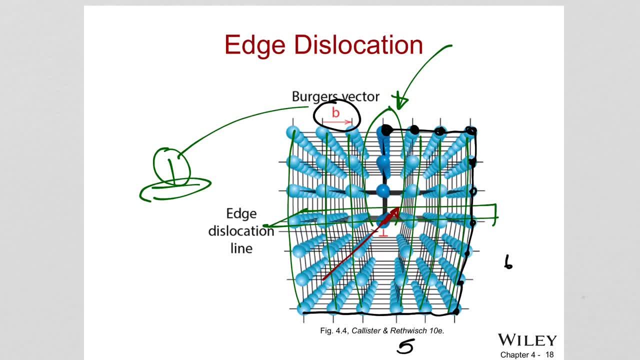 And I need to move 6 here for a perfect lattice to happen, Right. So for the perfect lattice I need to move in this corner also 5.. But I already walked 1,, 2,, 3. Right. 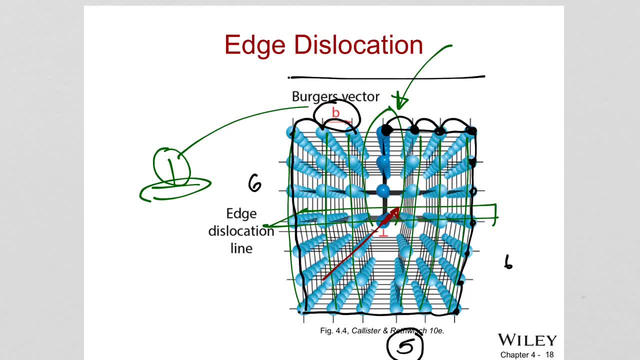 So 4, 5. Okay, But now if I want to complete that circuit, right Okay. So if you connect this finish to the start point, it is going to give you your Burgers Vector And 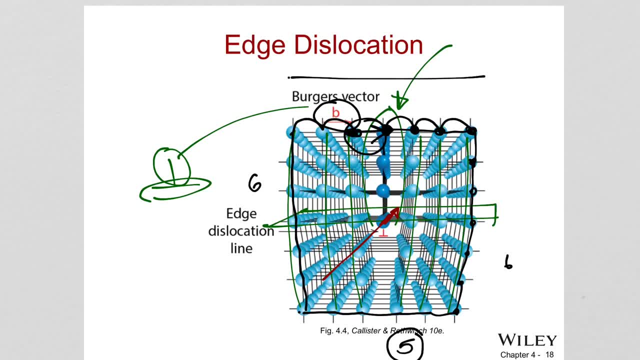 Burgers Vector is, as you can see, it's one atomic separation. Okay, So what I did was just I started from in opposite directions And when I did it, there was extra, extra atomic separation distance, which is: 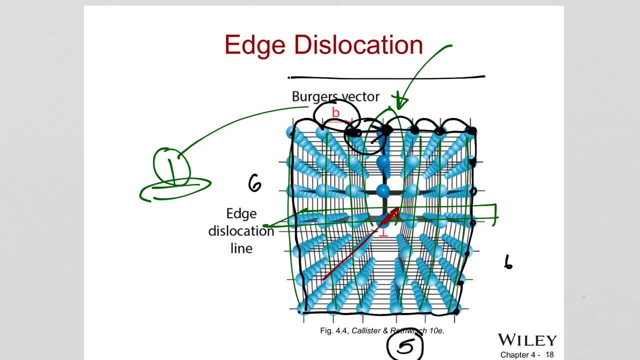 needed to be completed, And it is completed with the Burgers Vector, And that is giving us the magnitude of distortion. It is one atomic separation. Okay, That's it. So what we were concerned here, to understand this thing. 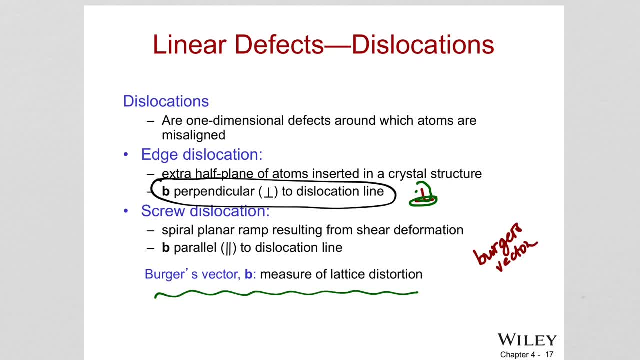 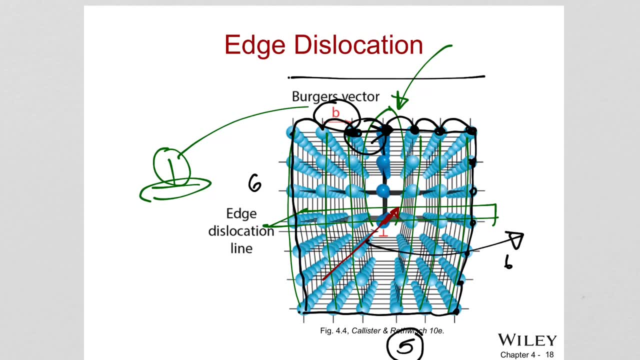 here, right, So the Burgers Vector perpendicular to this location line, So our dislocation line is this red one, right, It is getting. we are getting into the surface, to the screen, So into the screen, into the. 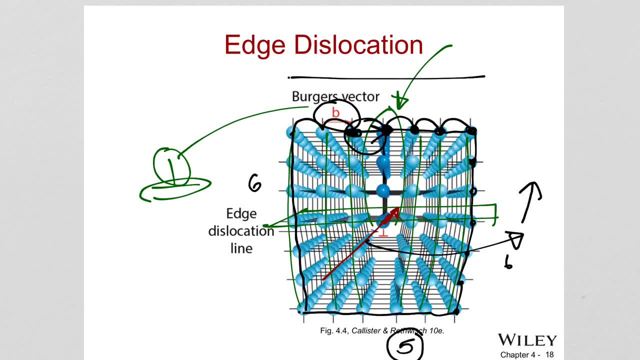 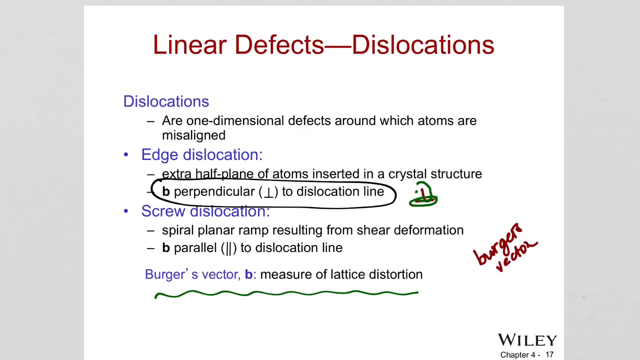 surface. It is getting towards inside, Okay, So of course that is the dislocation line that we cannot see it. Okay, Dislocation line is there, This is dislocation And this, of course, we can see. 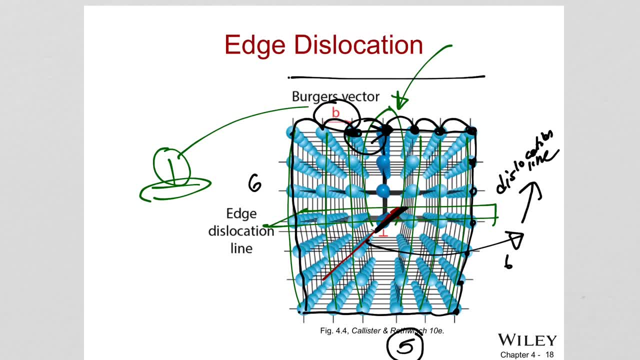 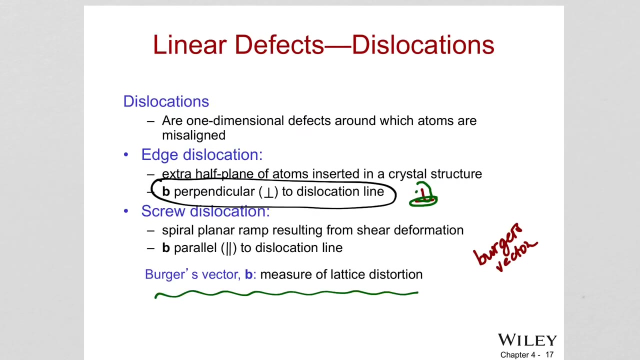 it is perpendicular because the Burgers Vector in this direction, right In this direction, or that direction, doesn't matter, It is perpendicular. perpendicular to the dislocation line. Remember, this is going into the surface, Okay, So, 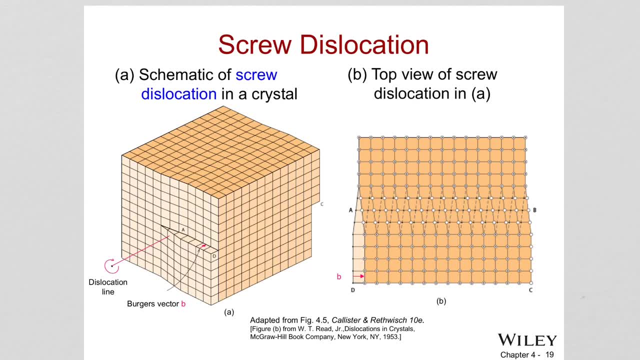 we understood that. right Now let's look at screw dislocation. That's a little bit difficult, compared to that, to understand. So basically, screw dislocation is formed by shear stress And this plane here going inside you. 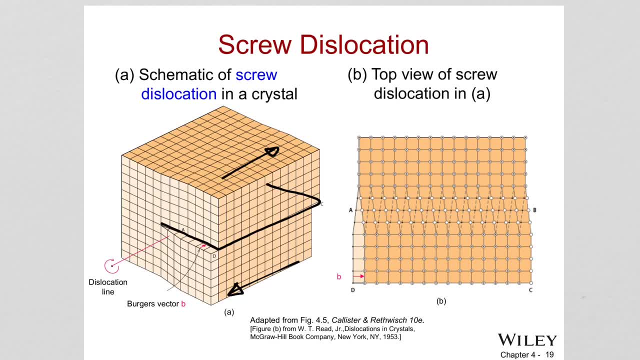 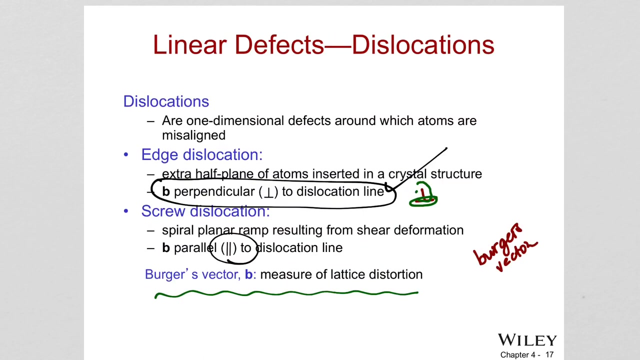 cut it, sliced it over there, the whole lattice, And when you apply these shear stresses, basically there is a shift in the lattice. Let me erase this. So where is the slope? Remember, in this case, parallel to: 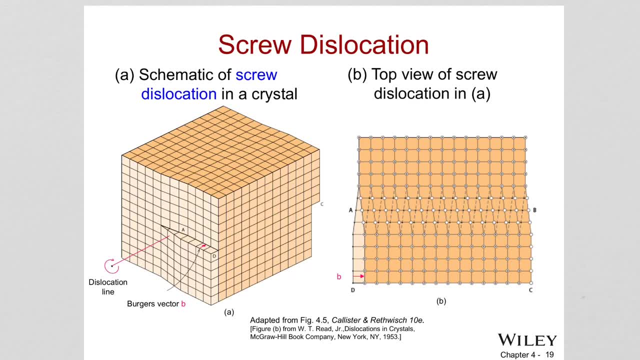 the burgers vector And the dislocation line is the line where this distortion happens. It is right there. Okay, This line is again going inside this structure And let's see where the how the burgers vector form. So let's. 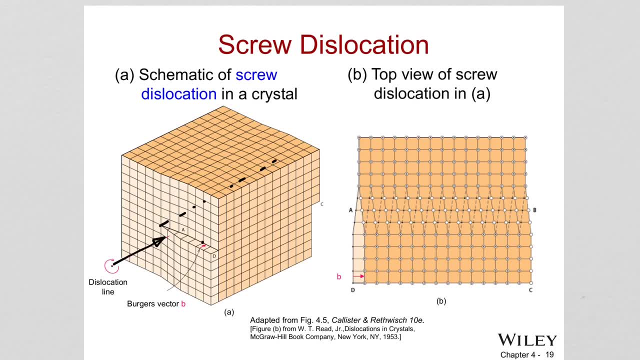 start from here And let's complete the circle right: 1, 2,, 3,, 4,, 5, 6,. 1, 2,, 3,, 4,, 5, 6, 1,. 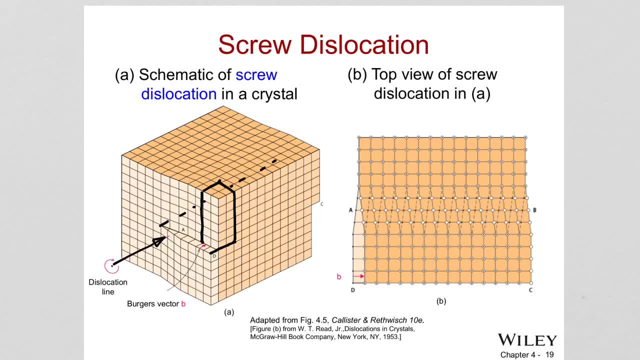 2, 3.. I need to move 3.. And then 1,, 2, here. So this is the burgers vector, right. So that is the direction and the magnitude is separation, And then 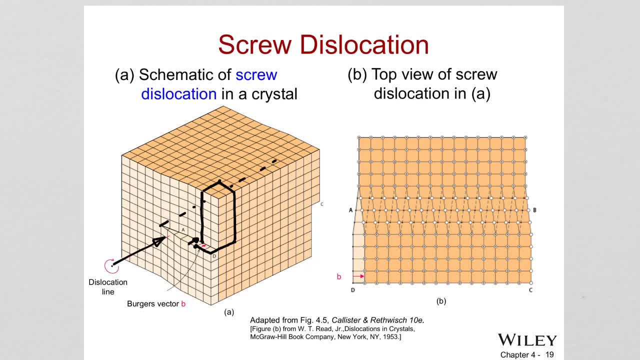 that's the burgers vector And it's parallel to the dislocation line, basically Okay, So that's the screw dislocation And this is if you look at from the top. this part is how it looks right. 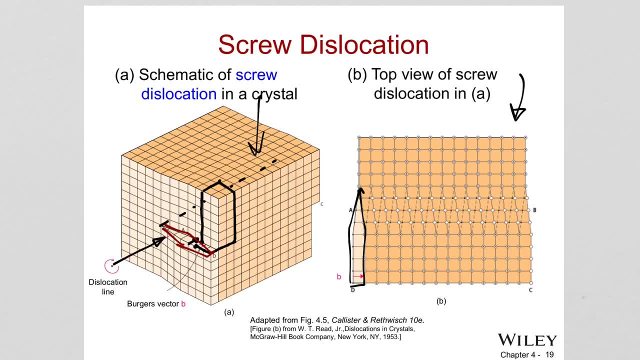 You see that how atoms are shifted, So normally this becomes here right- There's a shift distortion in the lattice along that line And dislocation line is parallel to each other. So if you guys having trouble visualization, as I 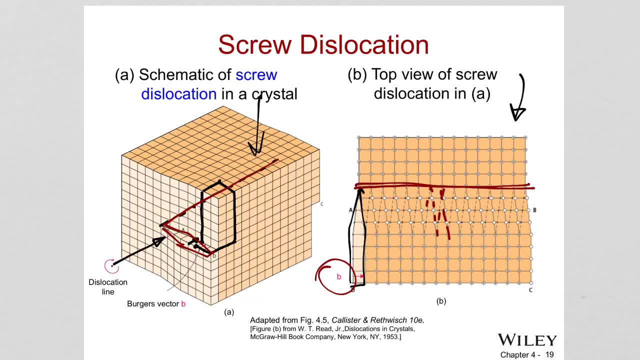 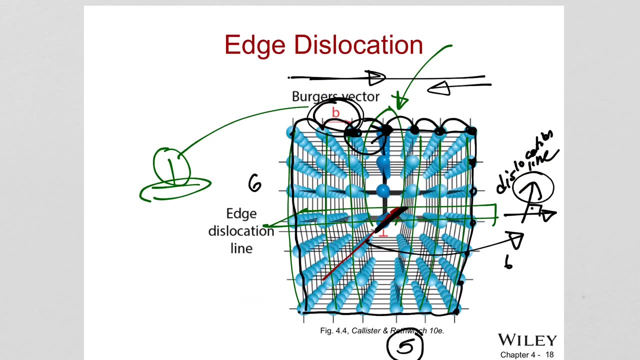 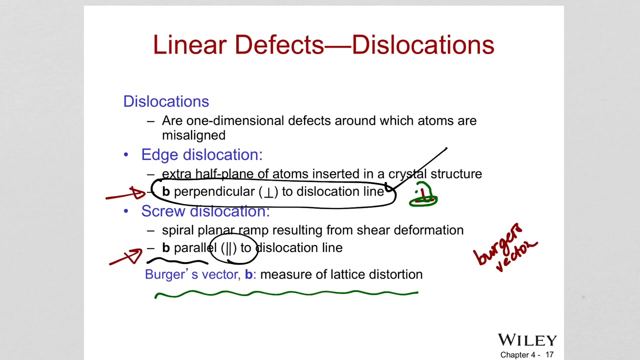 said, look at the images in the Google different views of this screw dislocation. I also sent you guys some YouTube animations for you guys to understand this relationship here, The relationship of the dislocation line with the burgers vector. that can be asked. 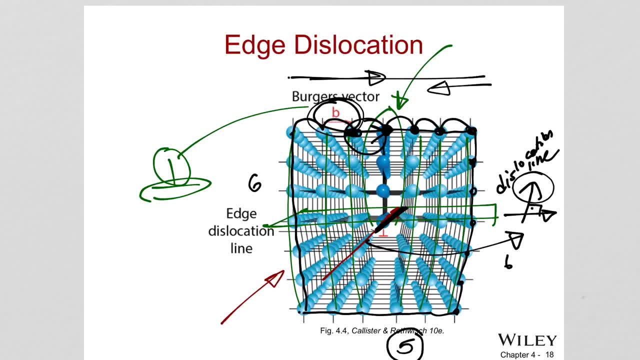 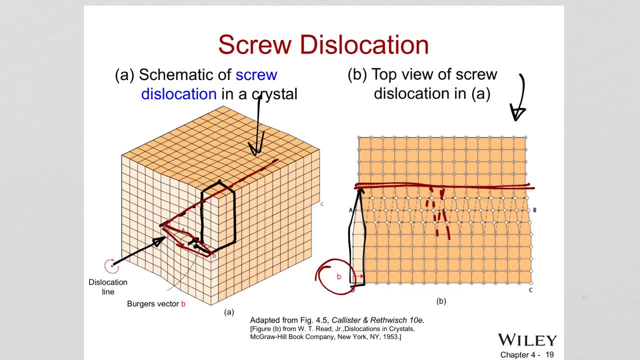 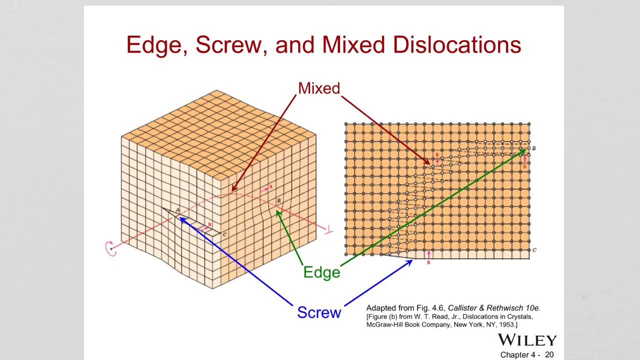 And I will also ask things like I will give you an image, for example, I give you this image and I'll ask you what type of dislocation line you see in the structure. So, in the structures, of course. 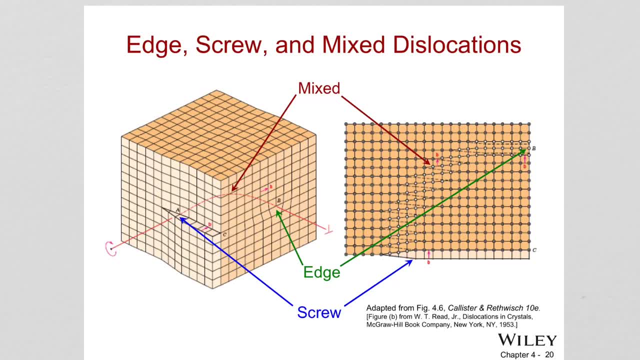 these line defects can come mixed like. it doesn't have to be a separate edge dislocation somewhere. there's another screw dislocation line but it is also mixed with the dislocation line of the screw dislocation that is happening there. So 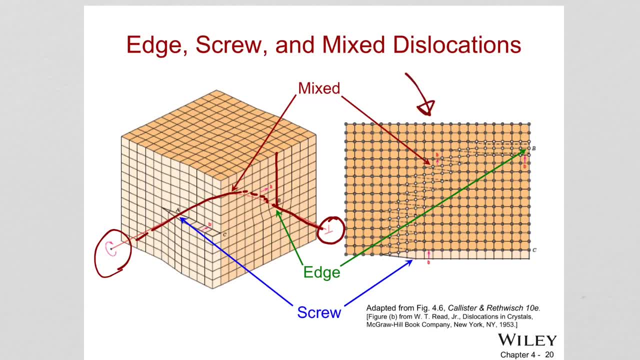 when they are mixed they are showing a difference in the distortion and you can see that here and you can imagine that. So there is some shift due to the dislocation. So those types of mixed dislocations are possible in the 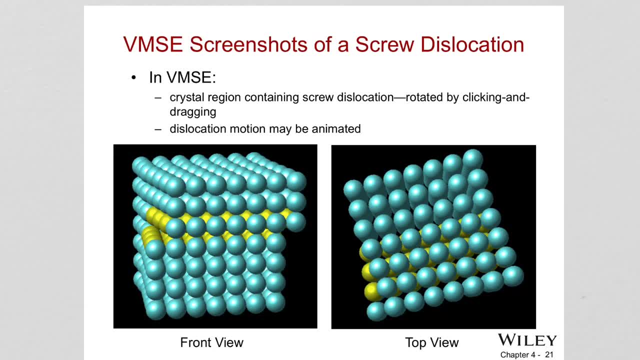 structure. So virtual material, science and engineering animations. I found this link and you guys can see it. I suggest you guys go there and there are a lot of animations, simulations for everything: for dislocations, for solid solutions, engineering. 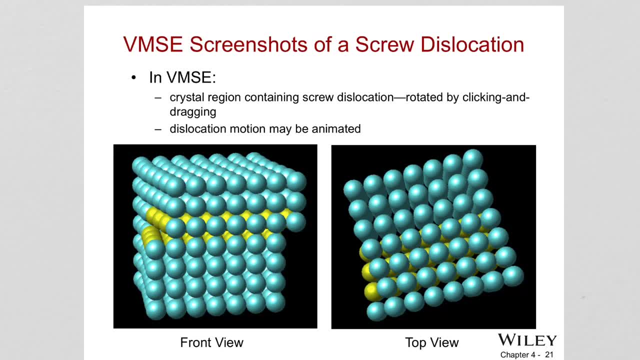 materials, crystallographic structures. I suggest you guys for the link. You guys go there and you guys go there and look at the animations, okay, So this is a nice opportunity for you guys to look at those. So 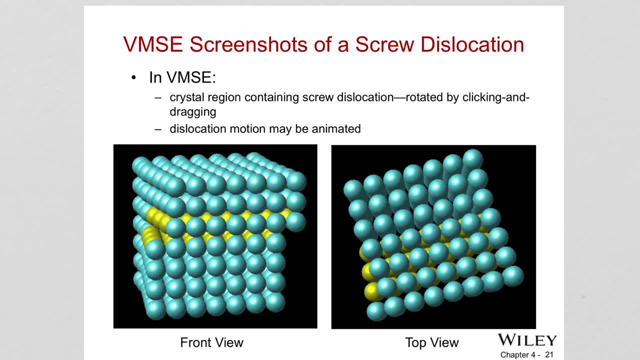 these are the screenshots from those animations showing you how you can see dislocations that are containing screw dislocations. This is from front view. this is top view And you can also see how dislocations move. Later we're gonna see that motion. 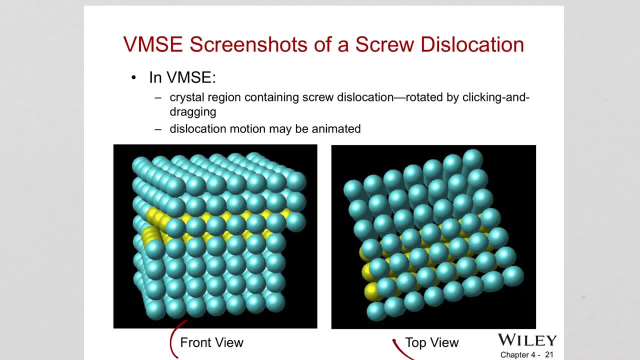 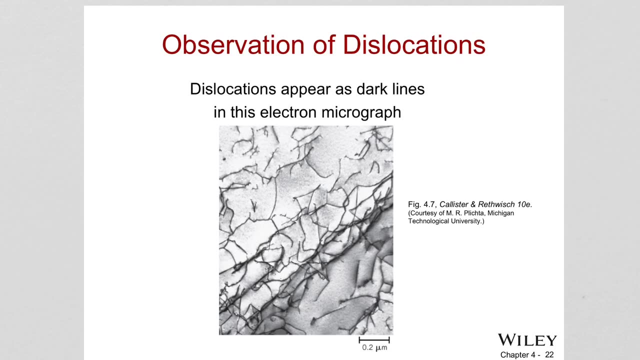 of the dislocation and how the dislocation moves and how the dislocation moves, So you guys can see how the dislocation moves. So this is a nice opportunity for you to see how the dislocation moves in the structure. So 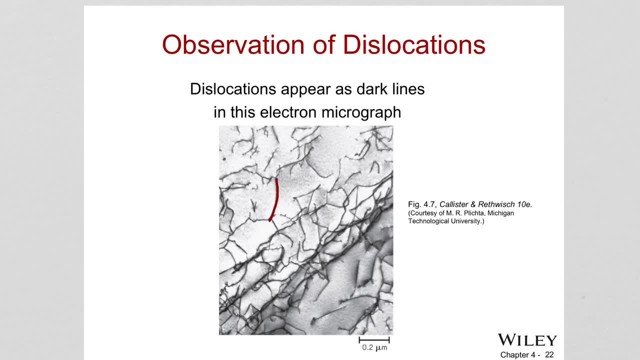 you can see how the dislocation moves in the structure. So you can see how the dislocation moves in the structure. So you can see how the dislocation moves. So you can see how the dislocation moves in the structure. 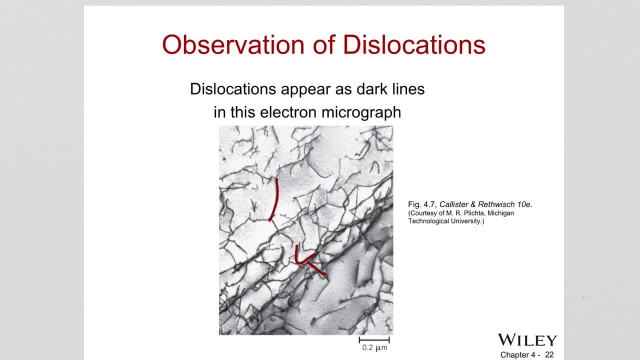 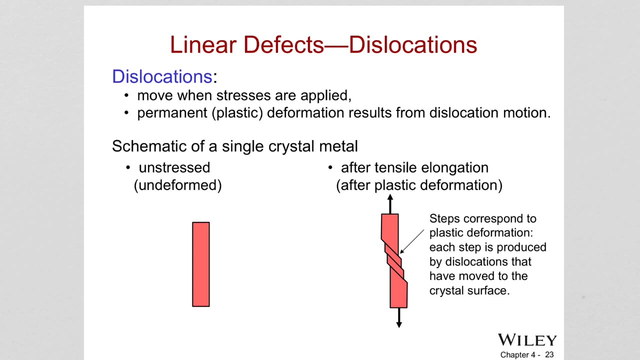 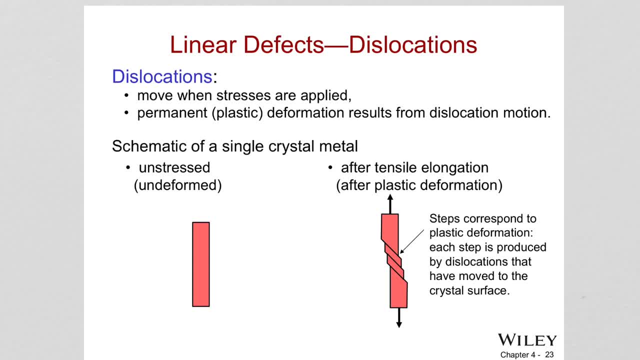 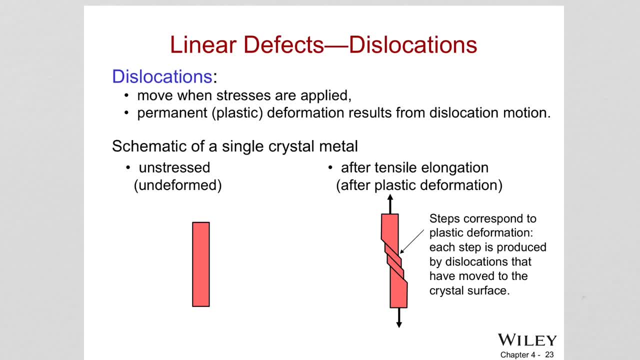 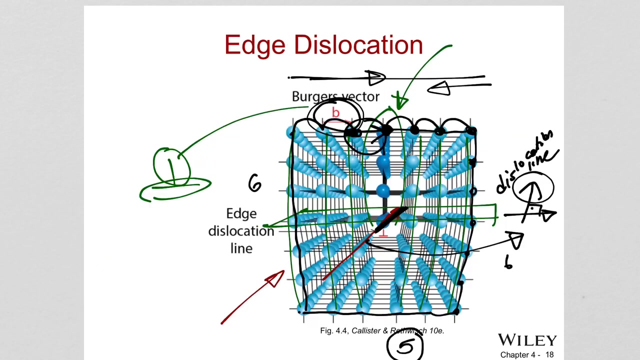 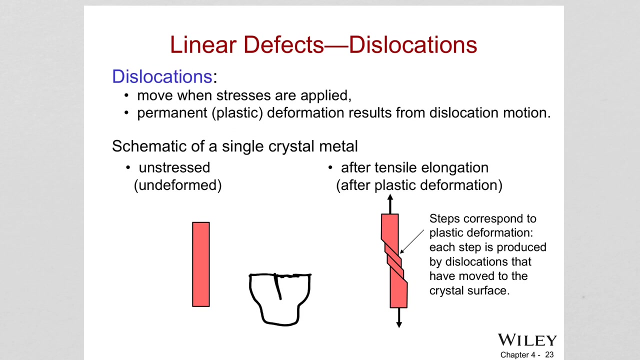 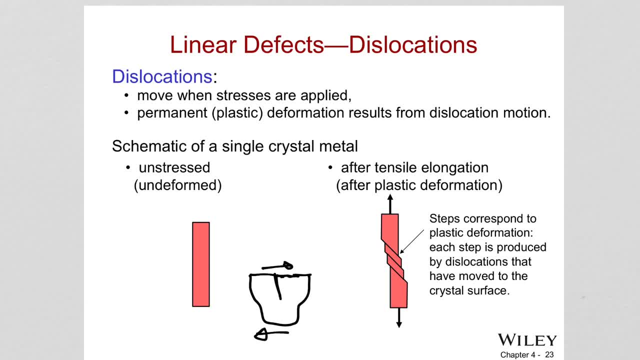 So you can see how the dislocation extra half plane of atoms go outside of the crystal structure. What you end up seeing is a deformed structure like that, Because one atomic distance the dislocation got at the surface, because that's where they stop. 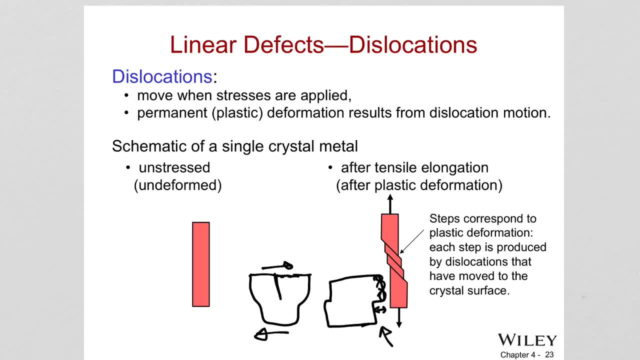 And, as you can see, for one dislocation moving, we are visually seeing that there is a change Of course. we are visually seeing because they're in the structure And when all of them moves and all of them reaches to the 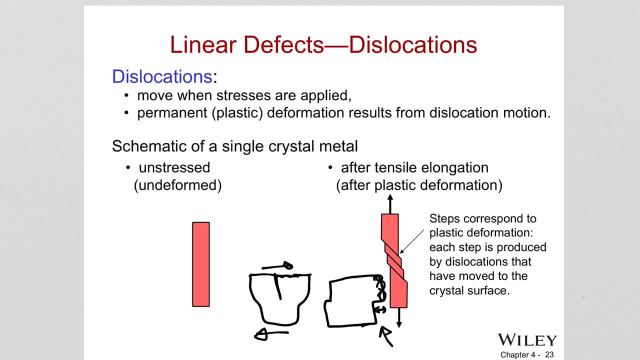 surfaces, there will be a macroscopic, visually seen change in the overall structure. The material will change its shape. Therefore, dislocations are the reason why we can shape the metals. If they don't have dislocations, we cannot shape the metals. 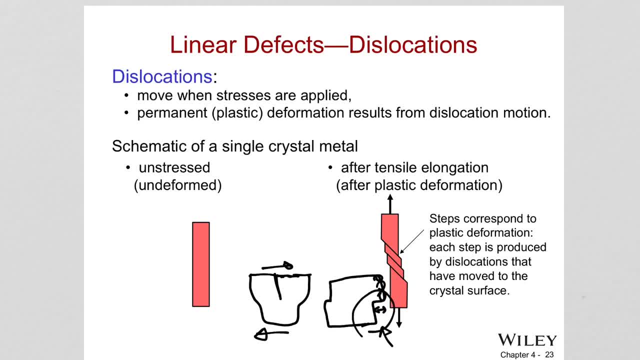 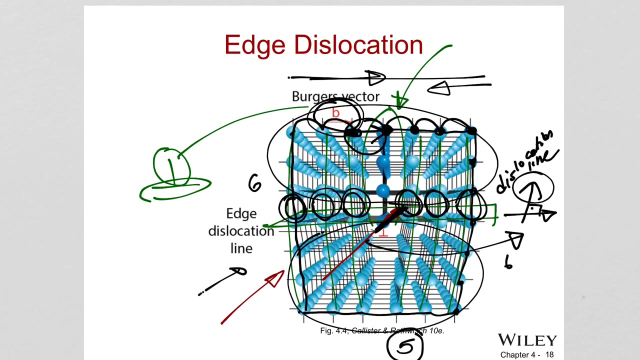 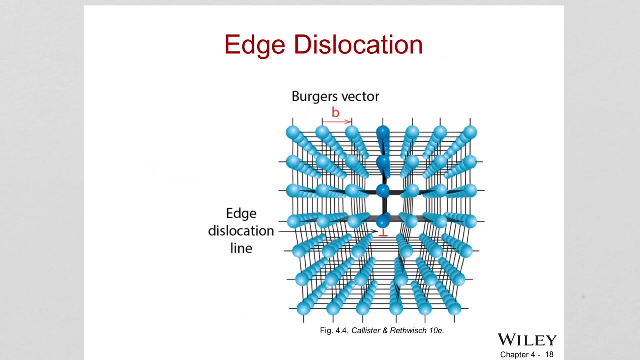 Okay, so I want you guys to look at the animation: dislocation, motion in the structure. So normally, why not? we just break all these bones here, Let me erase all these things, okay? So why not? just because we? 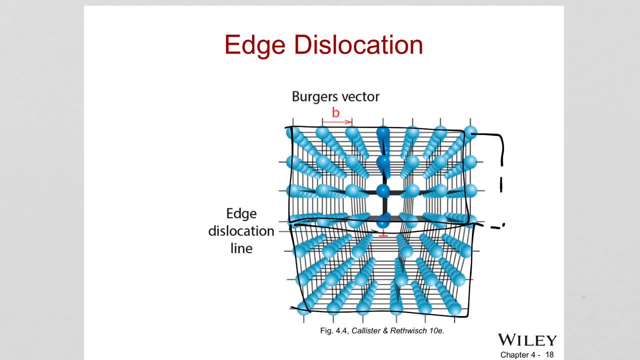 want a change like this? right, This goes inside. Why not just break all these atoms, all atomic bones? Just break all atomic bones and move the structure right. And that's why they did simulations to calculate the energy necessary to change the material. 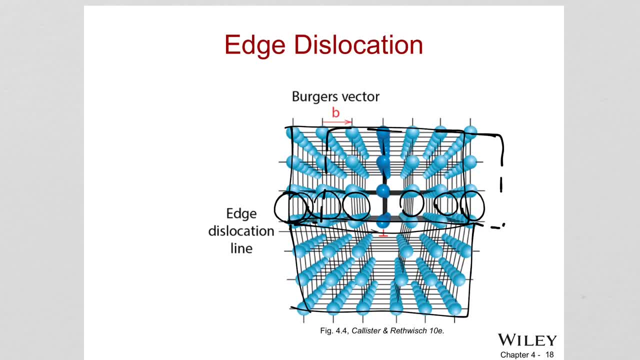 shape And they find these huge numbers. So why not break all these bones and shift the material layer by layer to obtain a change in macroscopically? So therefore, when they look at the experiments, though, it was requiring very little. 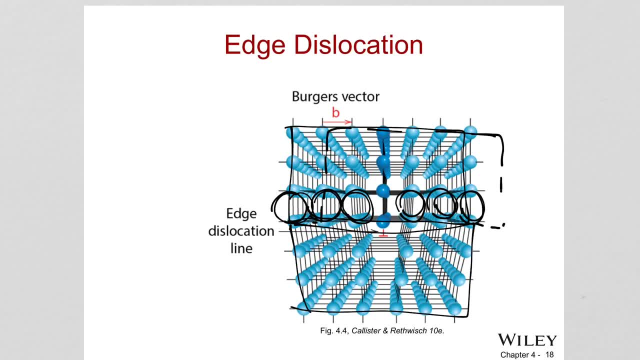 energy compared to the theoretical calculations to calculate the shape of the material. So theoretical calculations assume that in order to change the shape of a material we need to break all the atomic bones, But in reality, theoretical calculations assume that in reality, 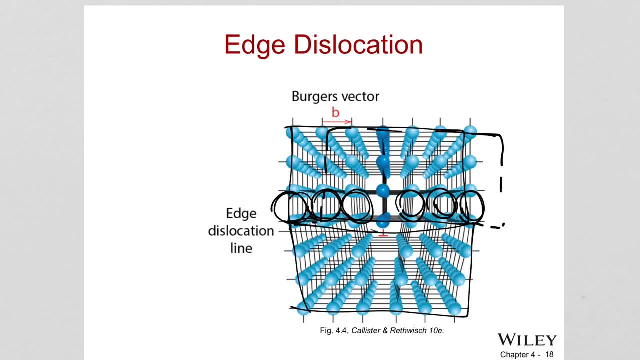 it wasn't that. It was because we have defects called dislocations, which requires much less energy to move in the structure that is giving us the permanent change shape. So it's easy for a dislocation to move, because it is actually not so. 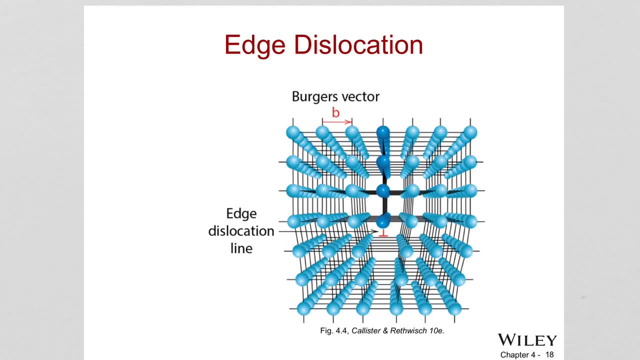 if you look at the animations, you'll see it is not actually this dislocation is moving, It is extra half plane and it's moving in the structure and there is only one single bond and this bond forms here. So breakage and forming. 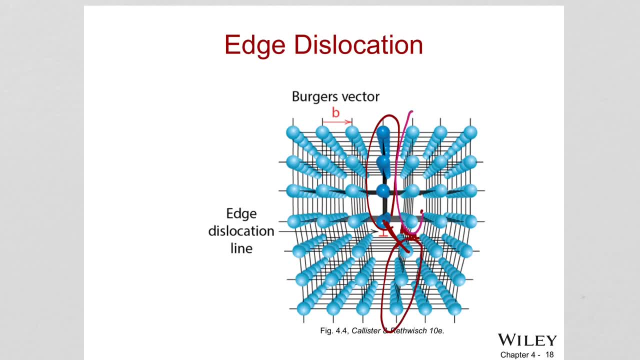 don't require much energy, Just one structure, then there, this will break, this will form energies compensated and this became your extra half plane of Adam. and this will break, this will form and this become extra half plane of Adam. and, of course, this, this much shift is 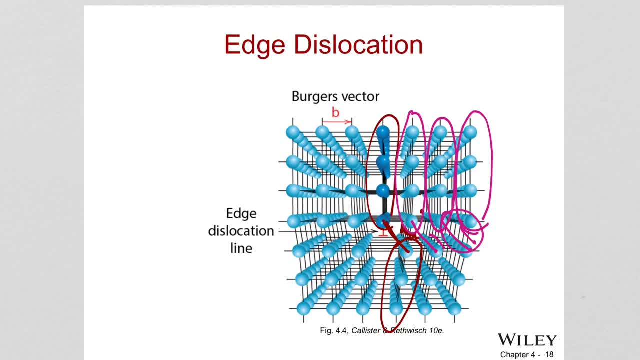 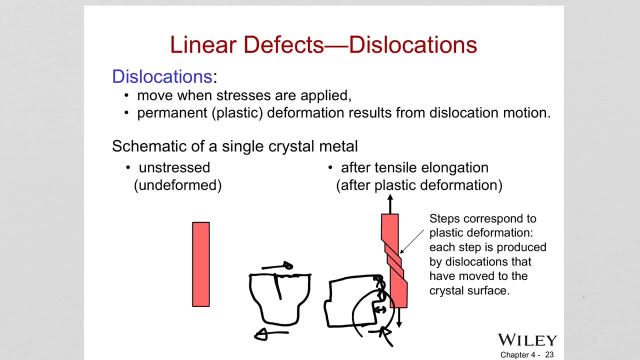 achieved in the structure. so look at the animations, please, and understand what I'm saying. and this is how the dislocation moves in the structure. okay, so, as we talked about this, if we have an unstressed meaning, there are no forces applied to a bar- let's say we apply tensile stresses and we see formation of 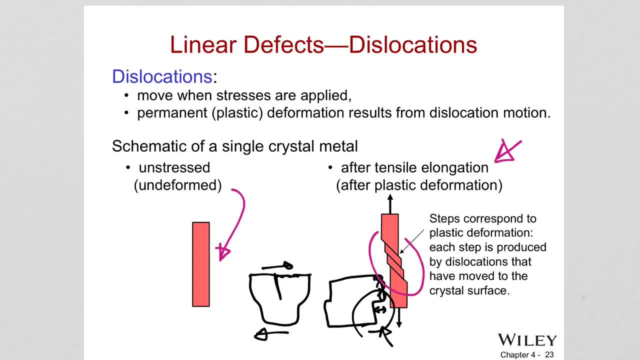 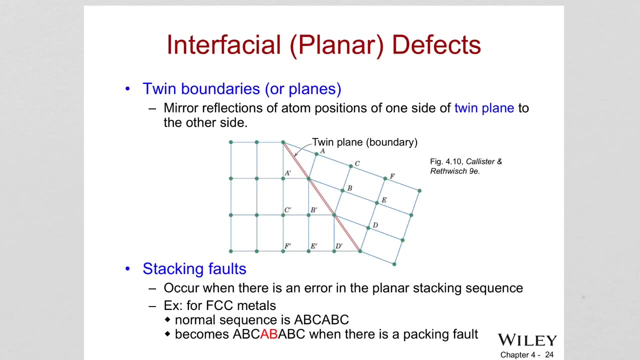 these tensile stresses and we see formation of these tensile stresses and we see formation of these planes, formation of planes sliding over each other. and, as we talked about, these locations are responsible for this permanent change, shape shift in the structure. so next is interfacial defects. these are boundaries that have two dimensions and 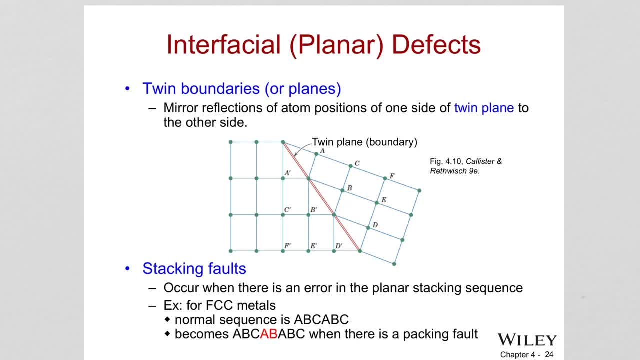 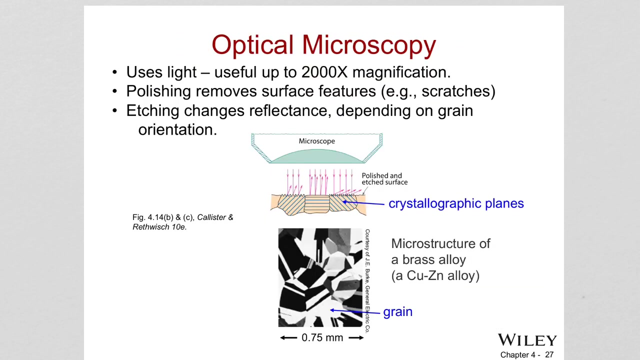 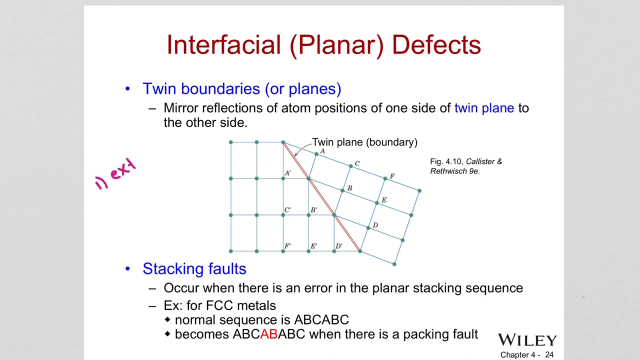 so next is interfacial defects. these are boundaries that have two dimensions and normally separate, separate regions of materials that have different crystal structures or crystallographic orientations, and we see that there are Examples are. let me see, let me write it down here. okay, Those are external surfaces to grain boundaries that I described in the beginning of this lecture. 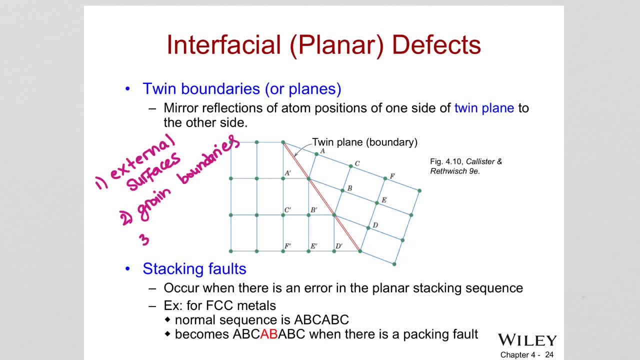 That's an interfacial defect. Three phase boundaries in between the phases. Phase is a region in space that has, in material space, different properties, different structures. If they have different, if you have different regions with different structure, different chemistry, those are different phases. 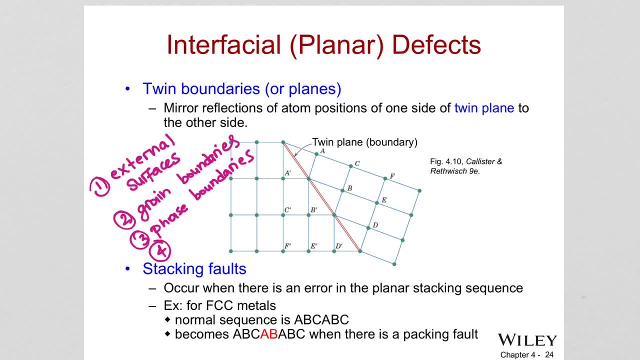 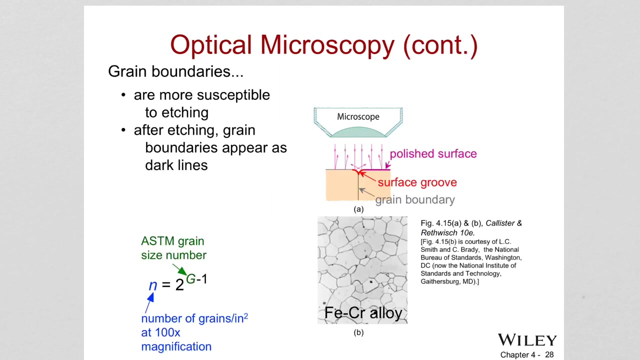 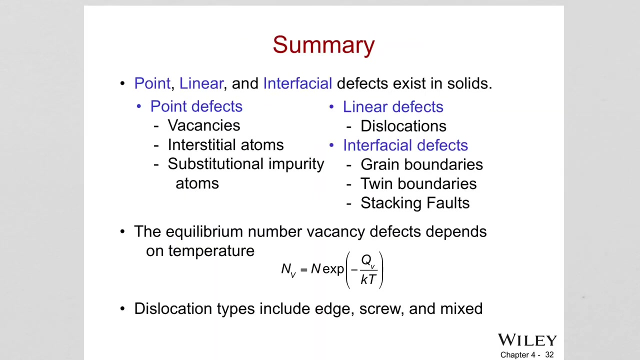 Okay. So four is twin boundaries And stacking forms. So we solved this one And I think now we're going to see external surfaces and twin boundaries and stacking forms, And then we're going to look at microscopic examination, different types of microscopes, And then we will be done Okay. 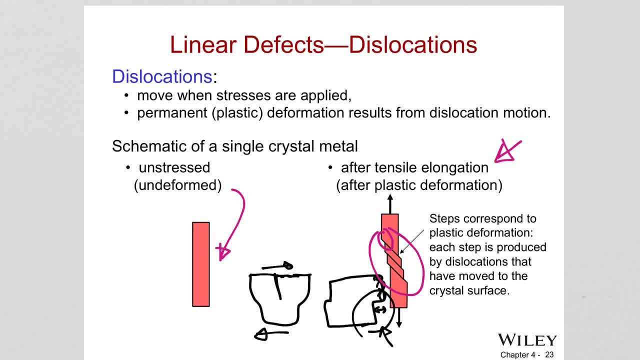 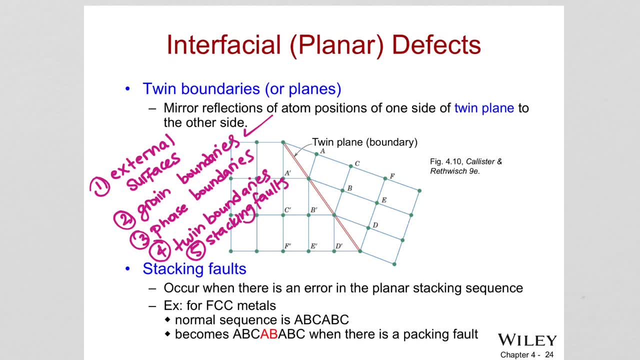 So let's see now what twin boundaries are. So the twin boundary is a special type of grain boundary across which there is a specific mirror lattice symmetry, That is, atoms On one side of the boundary are located in the mirror image positions to those of the atoms on the other side. 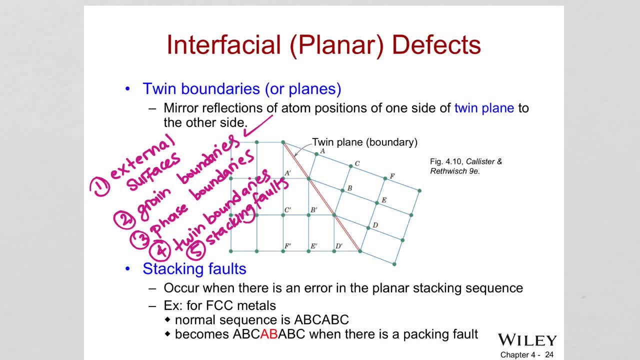 So it is like forming twin. So B is a mirror image, is B prime, D mirror image of D prime, E mirror image of E prime. So that is the called twin boundary. Sometimes this is the way And the refects, planner defects, form a special type of grain boundary, that is: 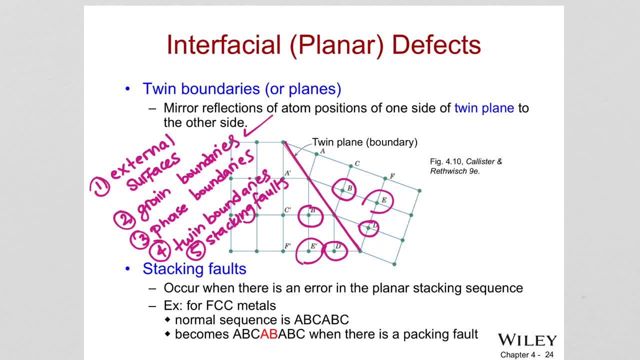 And actually this grain boundary is very important in the deformation also, Because sometimes beside the dislocation motion the twin boundaries can slide and also cause deformation. But this happens at certain times, condition: certain materials which we're going to discuss later on, later chapters. 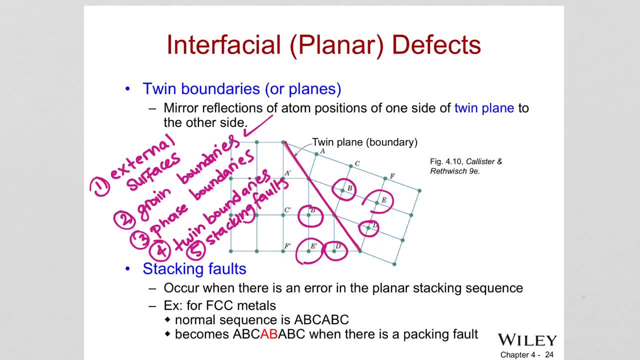 So basically this is just learned, that twin boundaries are a specific type of grain boundary where the mirror images of atoms form across the twin plane and there is also stacking folds. This is as the name implies. metals stack in different orders, right For FCC. we have seen that the normal sequence of packing was ABC, so A-plane, B-plane, C-plane on top. 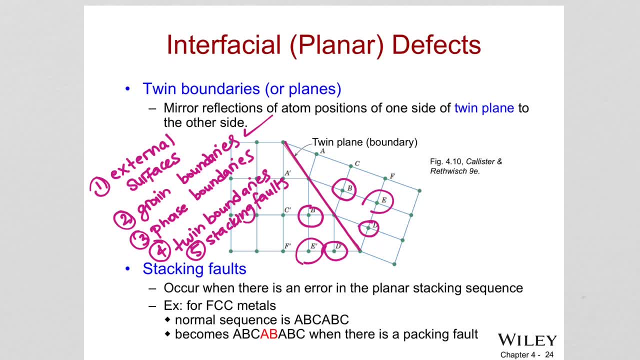 then A-plane, B-plane, C-plane on top. But if this packing is disrupted it becomes like ABC, AB, then ABC. like the C is missing, There is no ABC, There is no packing there. Then this is becoming a packing fold and we call it stacking fold. 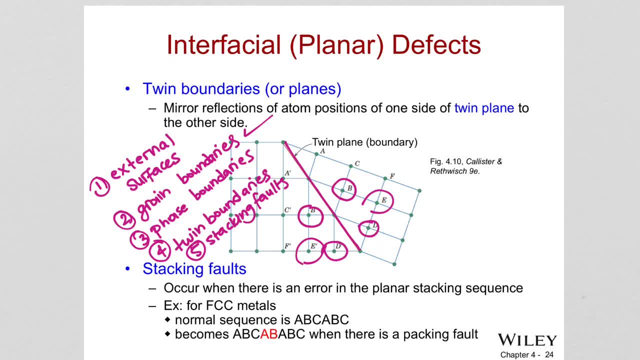 So there is going to be an amazing video link I will provide. Here you can see twinning, one form of plastic deformations besides slipping, And you will see that when materials deform, they deform by twinning, and this happens only in certain metals- okay, not all of the metals. 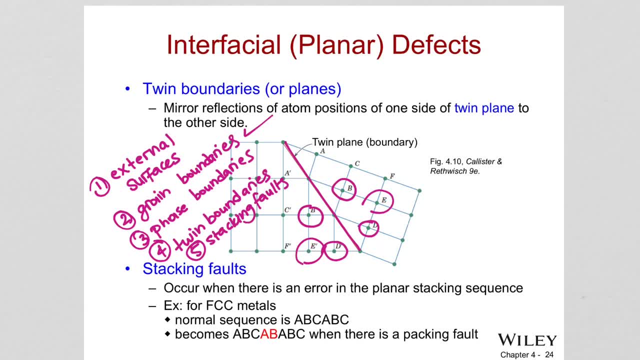 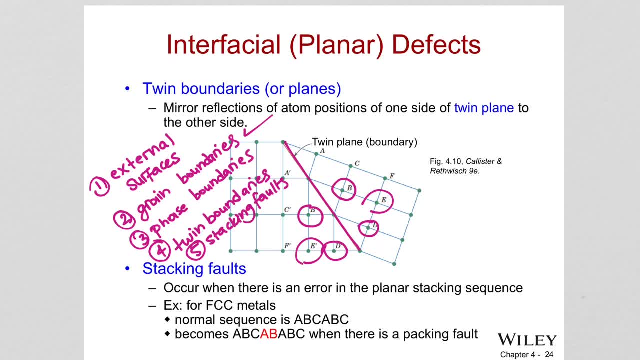 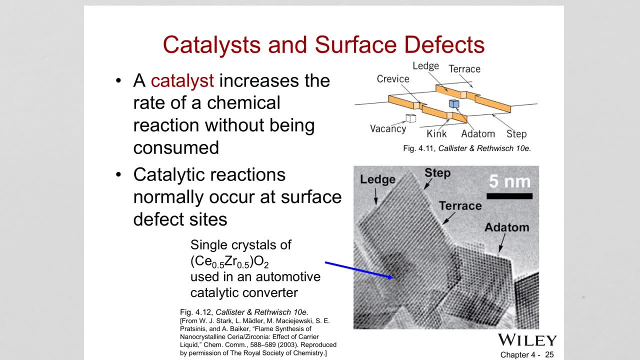 It is going to be. you will hear that noise and it is called tin cry. okay, It is going to be. you will hear that noise and it is called tin cry, okay, should watch it, okay, to see how thin cry sounds like. all right, so one another. 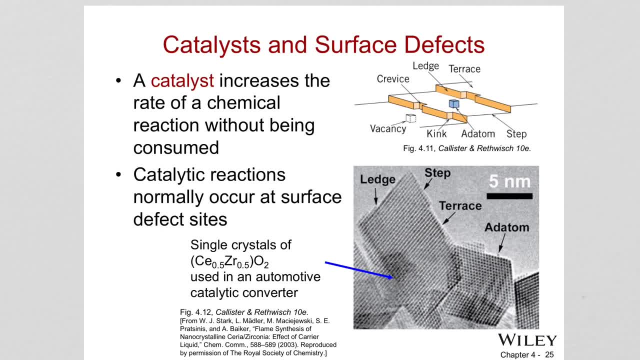 inter. another interfacial defect was surfaces right free external surfaces and we have seen that atoms so normally in the surface atoms, are more free, like this right, because within the bulk atoms are packed in an order where they are all surrounded with, in all directions surrounded with other atoms. but if you 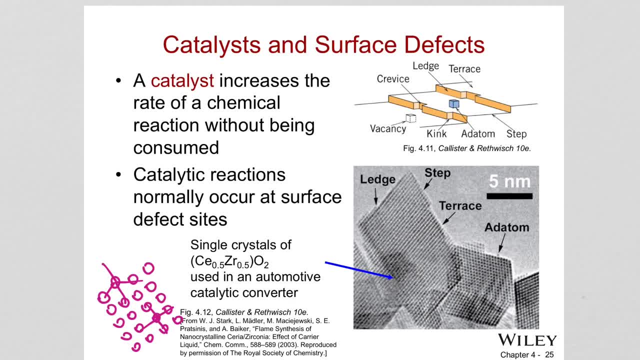 look at here- they are not surrounded everywhere- more free in the surface, right, and we talked about this- and it makes them more reactive, more energy, think they have more energy. they want to reduce this energy, react and 一起, Facebook nd Google Maps, give this energy and stabilize. Therefore these. 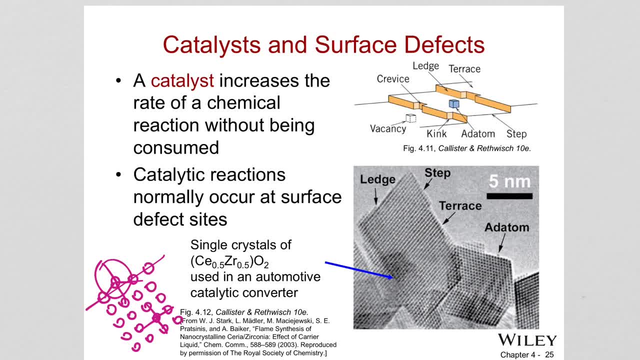 free surfaces where the atoms are more energetic can take place in chemical reactions as a catalyst. So a catalyst increases the rate of a chemical reaction without being consumed And providing surfaces to these reactions basically helps those chemical reactions to happen at a different rate, at a quicker rate. 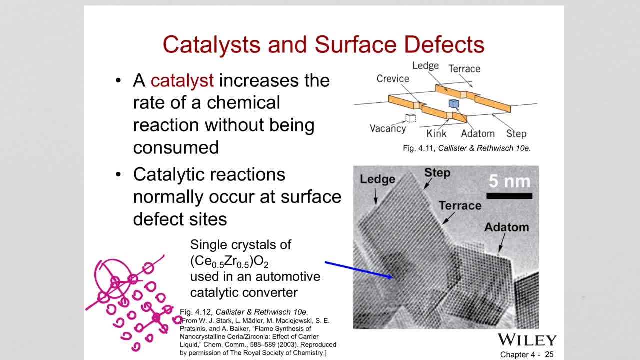 So in this example we are seeing single crystals of an oxide material which is used in automotive catalytic converters. In the electromicroscope image you see, we go to very tiny magnifications here and actually very high magnifications here, which means small sizes can be real. 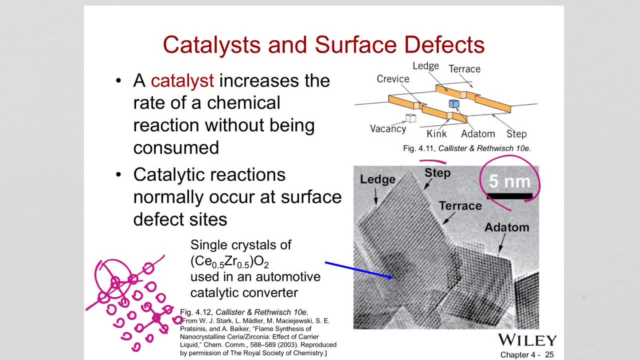 So we can see the atoms, Atom by atom. we can see how they are free. They are like they are not in an order right. They are more free at the surface. They are more disordered at the surfaces. We can see those. 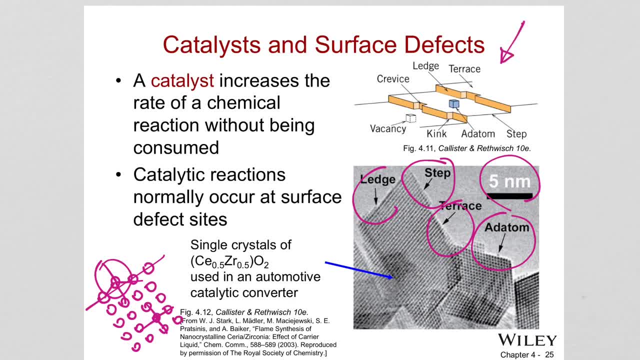 So in this illustration it also shows some representation of surface defects that are potential absorption sites for catalysts. These converters, the catalytic converters, are used to reduce emission of exhausts, gas and oxygen. These converters are used to reduce emission of gas pollutants. 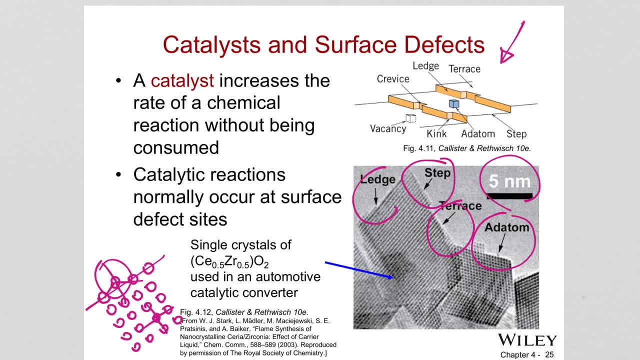 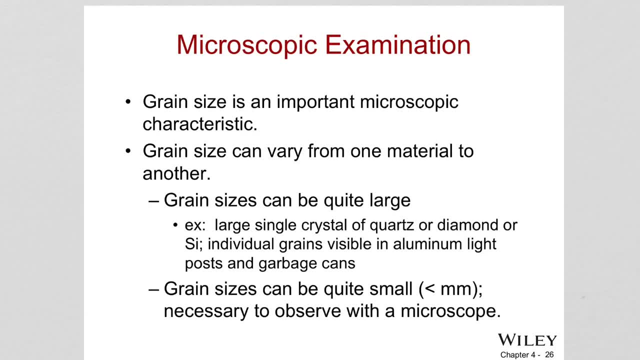 such as carbon monoxide, nitrogen oxides and unburned hydrocarbons. So actually it should be also described in the book. Besides those defects, let me go all the way to the beginning. Okay, I will pause it. 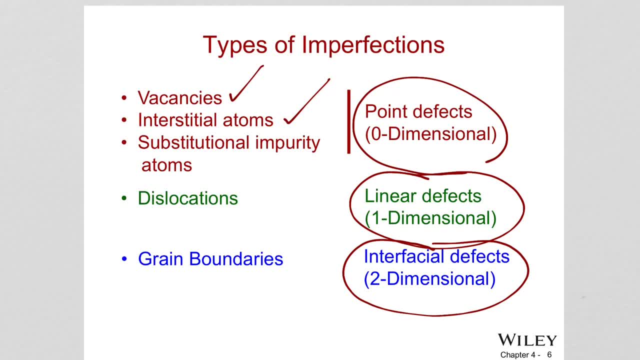 And besides those zero-dimensional, one-dimensional and three-dimensional defects, there should also be another defect that is mentioned and that is called bulk defects And this affects the overall macro. you can visually see like pores, cracks and what else, the things that you can visually see. that is affecting the whole bulk, the volume. 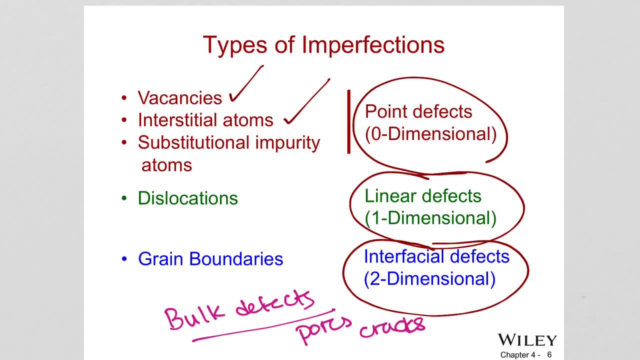 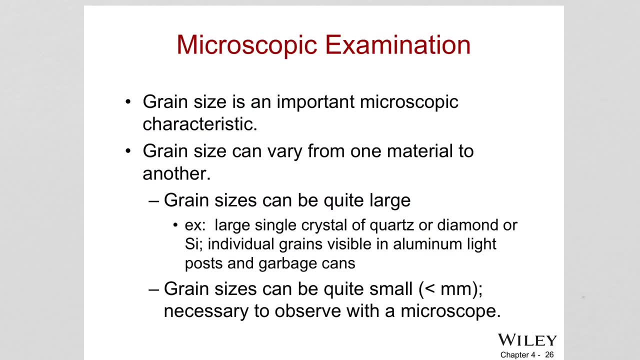 or you can see large defects. these are okay, So this should be also included. Okay, So let's now look at microscopic examination. meaning it is important you guys to understand how do we characterize materials? So these defects, how do we see? okay, 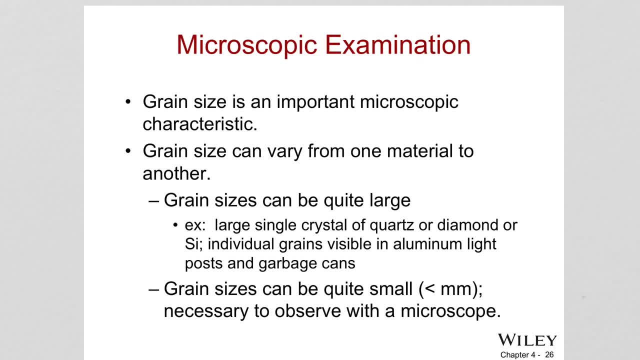 We are looking always under the microscope and there are certain types of microscopes. Not all microscopes will show you all scales, Okay. So if you want to see individual atoms, for example, right, you will have to do electron microscopy. or you just want to see micro scale, optical microscopes are enough. 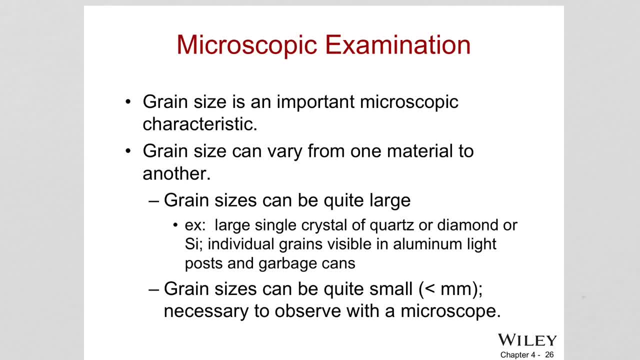 So in your book you're going to see, depending on the scale that you want to see, there are tables depending on the structure dimensions of the scale. Okay, Okay, Okay, So you can see all the structural features that you want to see. 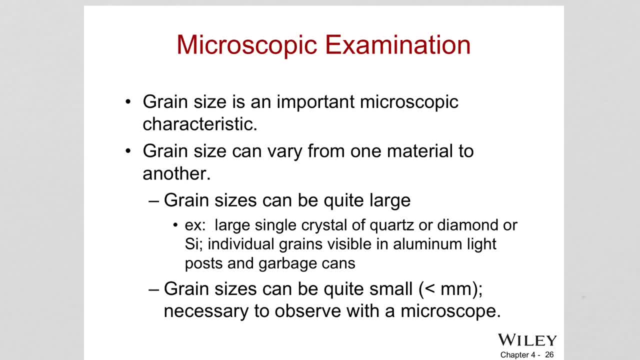 You can select which structural feature and then look at its dimension and, based on that dimension, you can see with which microscopes you can see those dimensions. Okay, There is a table, there is a bar chart that you can look in your book and read through. 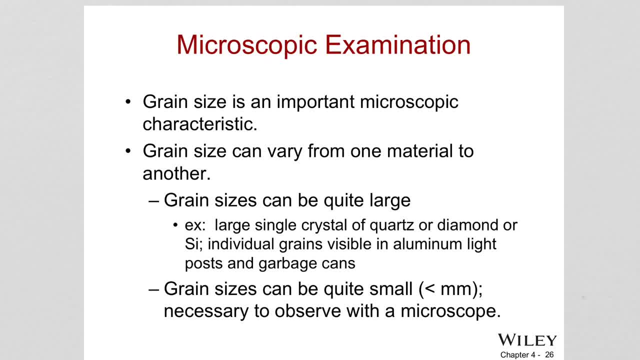 it. Okay, So in this case, we're going to talk about the micro scale, Okay, Okay, So we're going to talk about grain size, and how can we view this with the grains, with the microscopes? Of course, there are other features like atoms, unit cells, dislocations and grains voids. 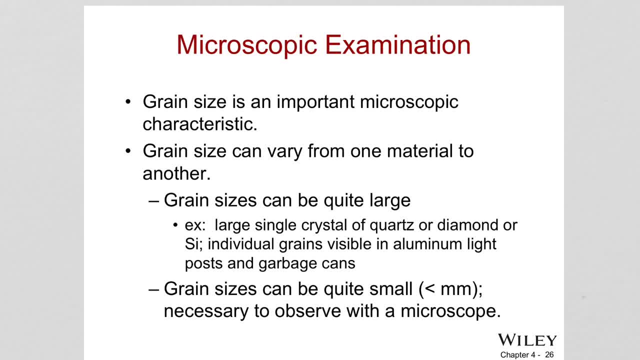 and cracks. Each will require a different microscope, and so grain size is an important microscopic characteristics, And it can vary from material. Okay, So if you see one material to another, they can be large and they can be small. They can be visual with the naked eye or you can need a microscope to see them. 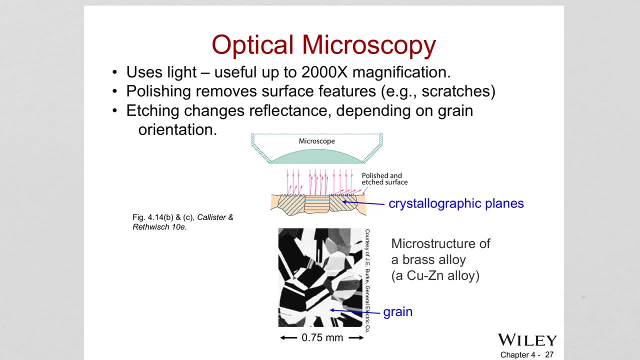 So one microscope we use to view grain size and grains is optical microscopy. Optical microscopy uses light And it uses magnifications up to 2000x, Meaning It magnifies 2000x. And to prepare your material to view under microscope, optical microscope, you need to 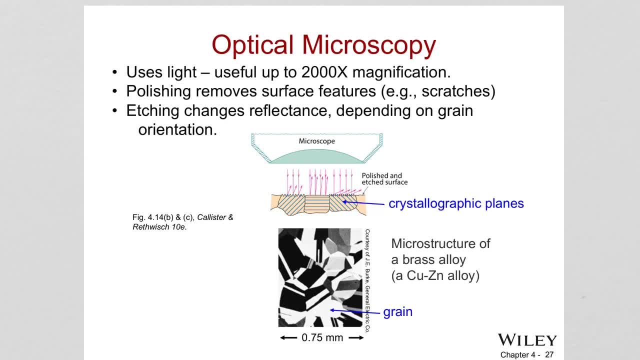 prepare its surface And this is done by polishing and etching. So polishing by mechanical means, polishing, we remove the surface features like scratches, And then we might need to etch, And I am using an acid. I explain to you guys: grain boundaries react differently because of their orientation. 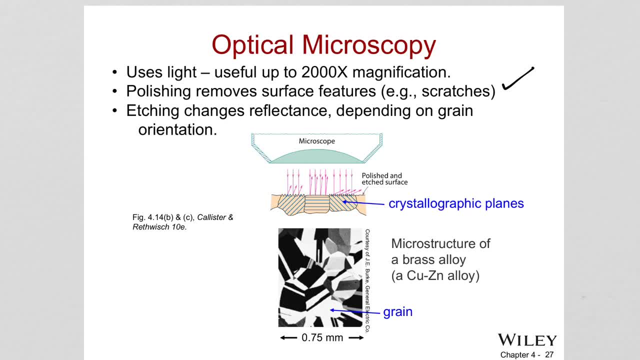 is different: more freedom of those surfaces. Depending on that, the different features will etch differently with the acid. That will affect what. That will affect the reflection of light, Because the microscope is sending light Right, Right, Right Licht zu überlesen. 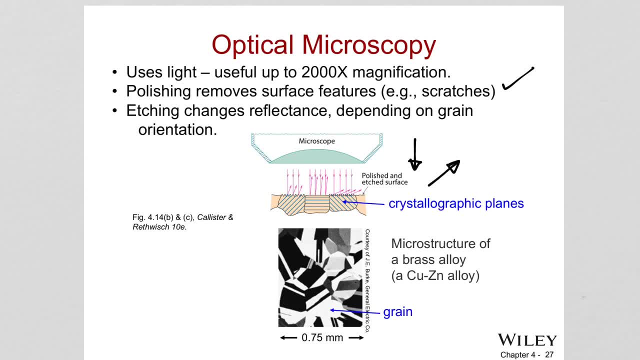 will reflect different directions. it will either come back to you. when you see a light grain under microscope, like this, that means the light is coming back to you, and then, if it doesn't, for certain grains. you see, at certain grains, atomic orientation is different. of course. this difference, 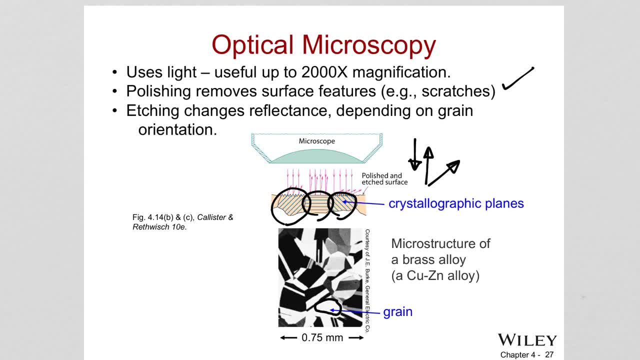 in atomic orientation will change how the light is reflected, and so some grains will reflect light back to you, some will reflect it away, so you see them as dark regions here, dark regions, right, and some of them will have an angle, so you might see gray, and this is how the grain structure. 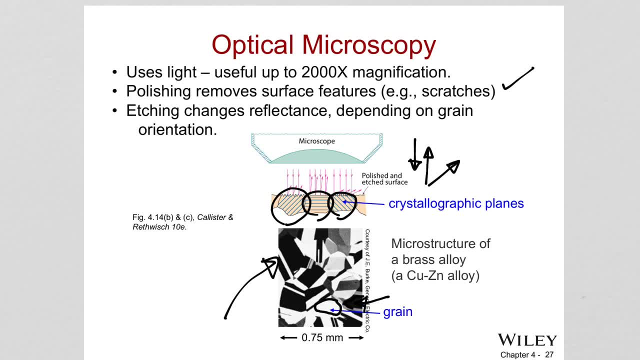 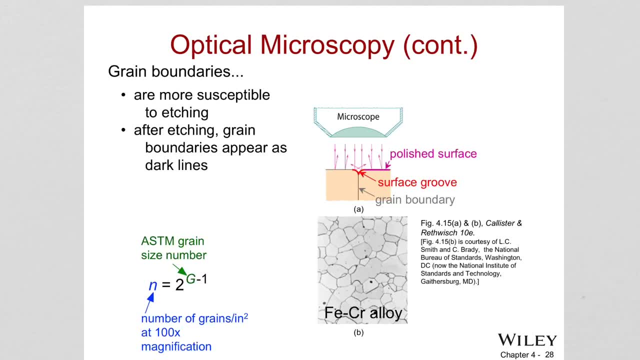 will look like under my optical microscope. this is an example for a copper zinc alloy. so that's what we talked about initially in the class. in the lecture i told you guys grain boundaries. they are more susceptible to reacting with acids during the etching and they appear as 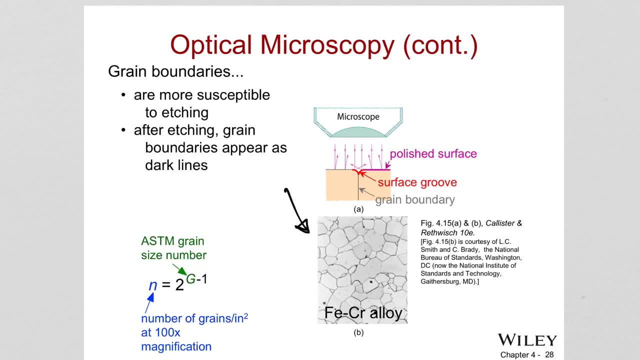 dark lines. they exactly show the example i discussed with you guys. you see the polished surfaces and surface groove forming because there are grain boundaries. those places are etched differently are at because they are more reactive. when this happens, they scatter the light differently, as you are seeing here. and then, based on those microscopic images, 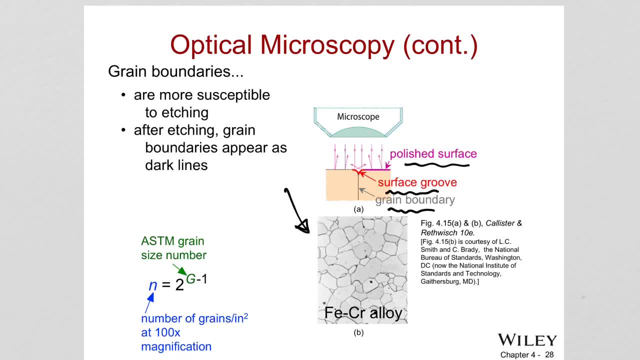 people come up with a common technique to calculate the grain size. this is done to characterize materials based on their grain size. they can say: for this application, i need a material with a grain size of eight. or for a sheet metal, for a car body, i need a grain size of this for this. still for this metal alloy. 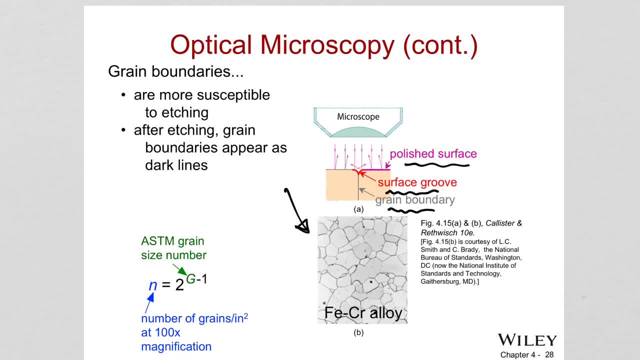 so they wanted to characterize materials or give them names, give them preferences based on the, the grain size, and therefore American Society for testing in materials come up with a calculation of grain size number and the grain size number is G and the formula is given this way: 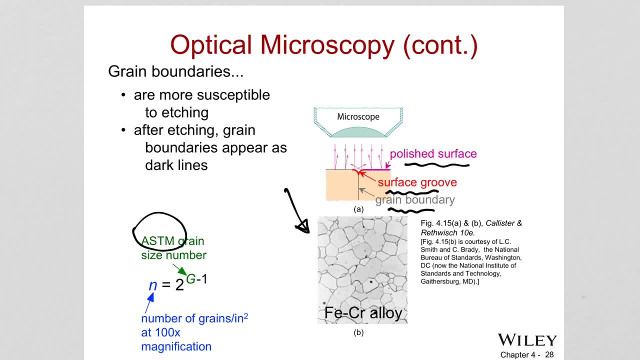 So what you need to do: collect a microscopic image and in this image get an area of one inch square. so one inch, one inch here, one inch here. this makes one inch square. so let's say, one inch square here, one inch, one inch, and then this is has to be done hundred X. 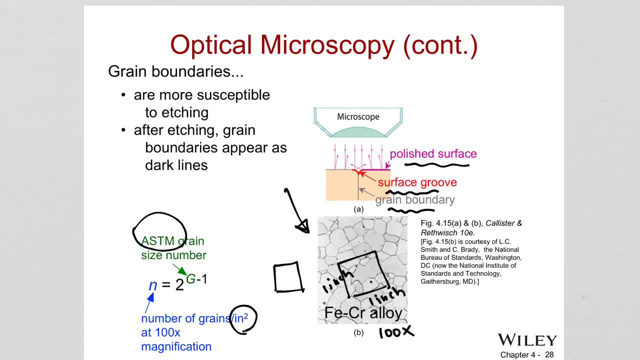 so your image has to be at hundred X magnification, for of course this is a standard technique, so you use it for every material. that's the way to we can compare different materials. there are Right. so get the image- microscopic image- at hundred X and find area that is one inch. 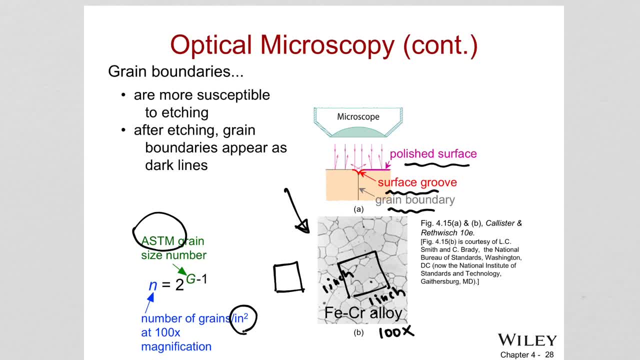 square within your microscopic image and count the number of grains and this is represented by the number and this and is giving us the number of grains in per inch square at a hundred X magnification. and when you put that information in this equation, That you obtain a volume for G and that G is given you, giving you the grain size number. 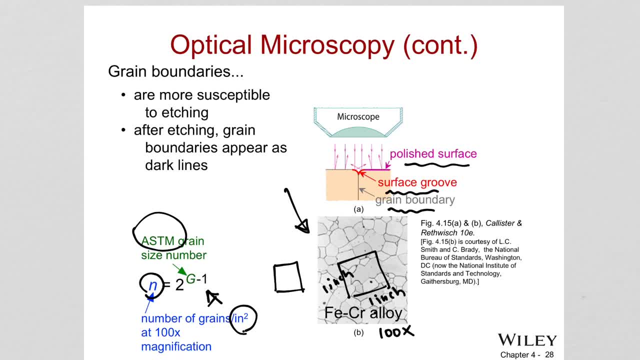 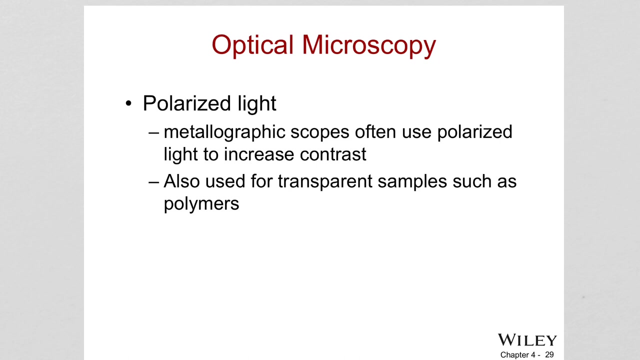 that is used to compare different materials because grain size is important in determining properties. Okay, so they wanted to separate, categorize material based on their grain sizes, So I will upload one problem regarding the Grain size. you guys should check the notes, okay, So sometimes polarized light is being used. polarized light, basically: you, there are light. 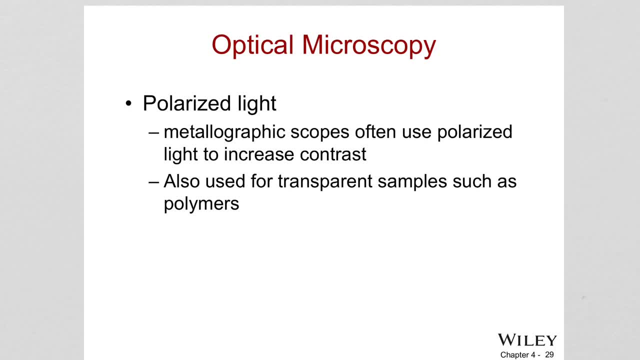 has different vibrations, different direction vibrations, and if you polarize it, for example, you can only let like filtering It. okay, only vertical vibrations to get past through, for example, and when that happens you can increase the contrast, and usually those polarized lights are used to characterize. 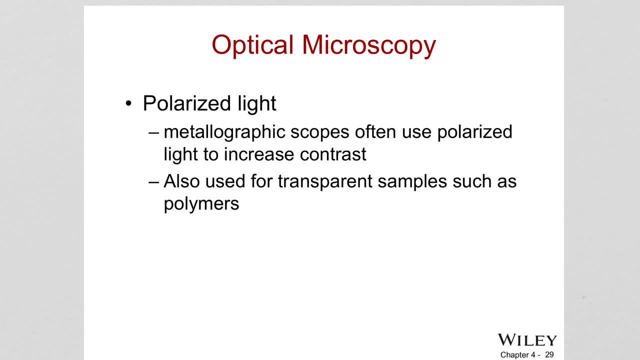 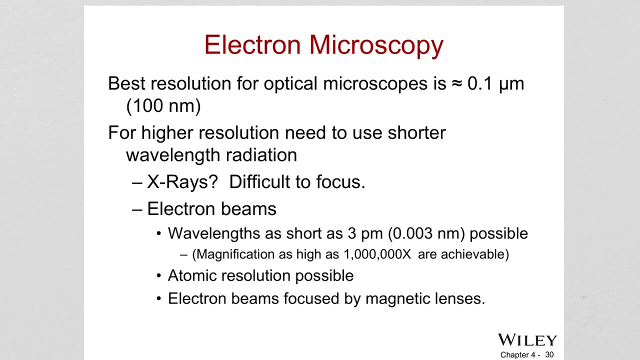 polymers. So when we come to the topic of polymers, we can see this in more detail, how they look under microscope. Well, electron microscopy has a better resolution and we can view more small features, smaller features compared to the optical microscopes. Okay, so around hundred nanometer, very tiny, nano scale features we can see. 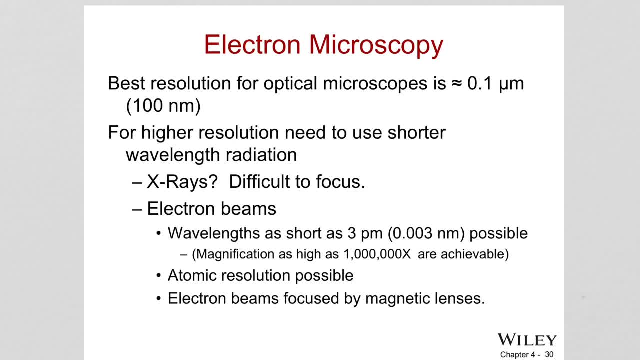 Of course, there are wide range of electron microscopes, so there are electron microscopes. even you can see the individual. So, instead of light, this is using an electron beams. okay, and electron beams is very easy to focus on one spot, because why you can use magnetic fields okay, normally optical. 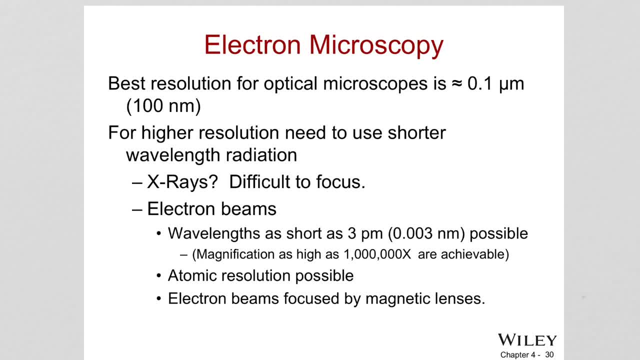 microscope, you use lenses to focus on the light in electron beams. you can own magnetic lenses to focus on the beams at certain point And then therefore get information from the light. Okay, Okay, Okay. To get information from the surface of the material. 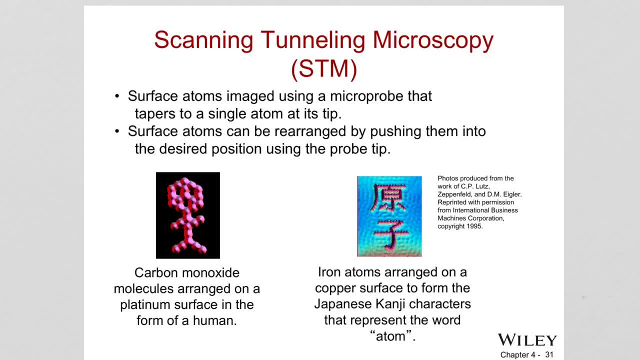 So scanning, tunneling, microscopy, this is when we look at the surface atoms and image them. So surface atoms image using a micro probe that tapped to a single atom at this tip tip. So there is a tip that is scanning on the surface, moving on the surface of the material And, of course, when it encounters atoms like think about, like the atoms are coming, like that right. 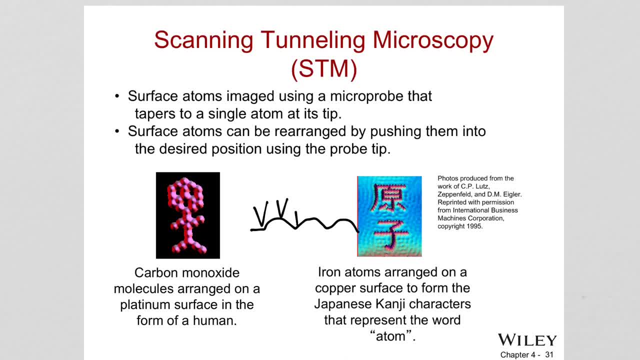 And this tip is scanning the surface, moving along the surface like that, Okay, And then of course it goes ups and downs. Therefore it detects information and then gives you an image of the atomic arrangement on the surface. So we are seeing here. they obtained carbon monoxide molecules arranged. 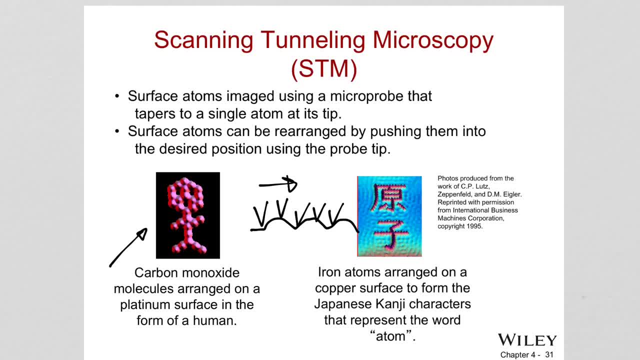 On a plutonium surface in the form of a human And some Japanese character. they were able to arrange the atoms in that form, Etc. So the basic idea here is: you can view the surface atoms with this technique And in the next video we will talk about the atomic arrangement. 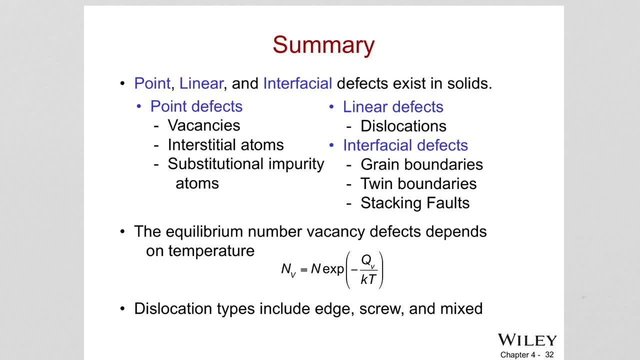 And in the next video we will talk about the atomic arrangement. summary: what we have learned. we have learned defects: point, linear, interfacial and bulk defects. point defects were vacancies, interstitial atoms, substitutional impurity atoms, and linear defects were dislocations, edge and screw dislocations. interfacial defects were grain boundaries, twin.